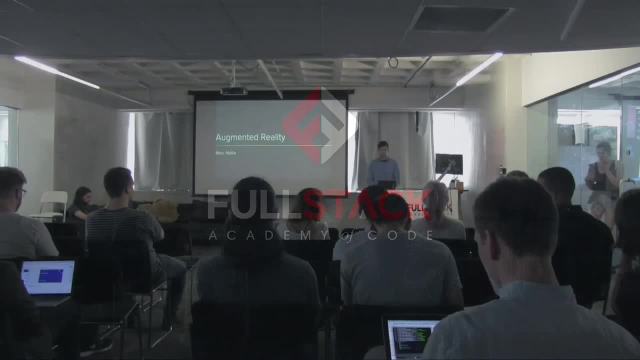 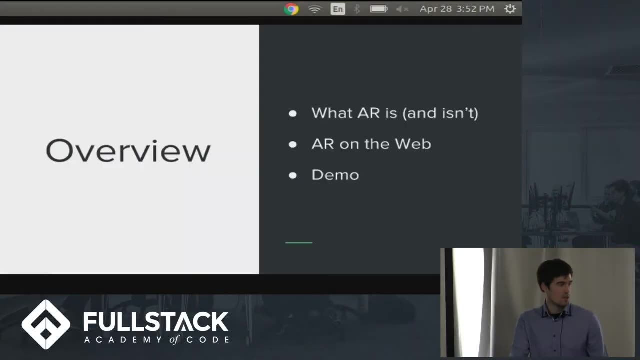 Good afternoon. my name is Mark, and today we'll be talking to you about augmented reality and how it can be implemented on modern web browsers. So here's a brief overview of what I'll be covering in this talk. First, I'm going to explain what constitutes augmented reality. 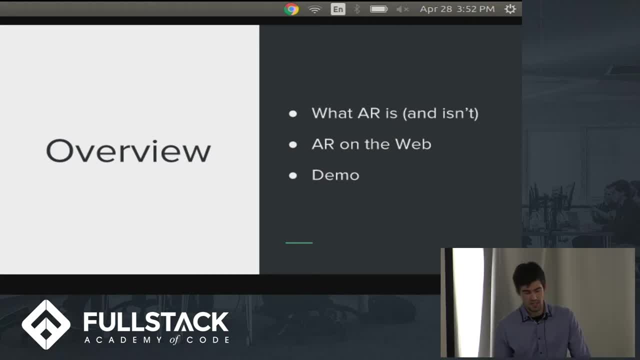 so what it is and isn't, how to make it, the different forms it can take and how you can interact with it. Next I'm going to go over how it can be implemented in the browser, and that's going to kind of transition into a relatively simple demonstration of a browser-based 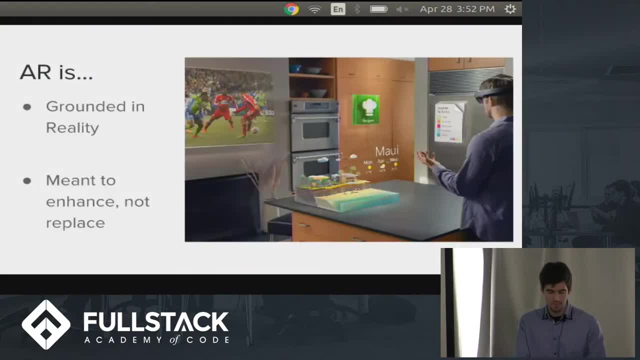 AR app. So let's get started. AR is pretty self-descriptive. It is augmented reality. The basic principle behind any AR interface is to analyze your current environment in order to project images or objects onto it. Ideally, you can interact with these objects. but it's not really a requirement. The way I see it, AR is that it's not really a requirement. The way I see it, AR is that it's not really a requirement. The way I see it, AR is that it's not really a requirement. 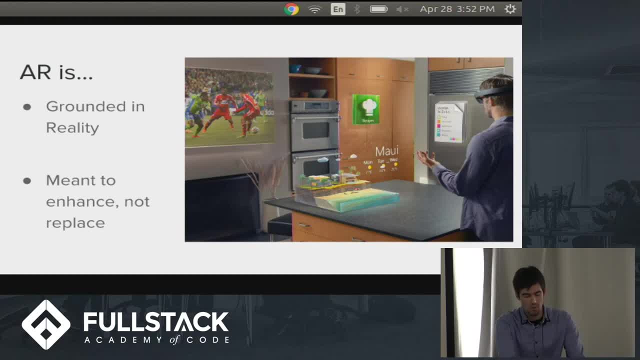 AR is meant to enhance your real-life experience by keeping you connected to the virtual world without really breaking from it, which is to say, you don't have to pause from what you're doing by grabbing a phone in order to check your updates, emails, messages or whatever. 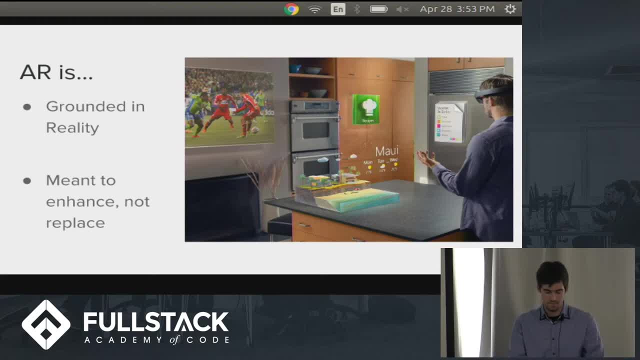 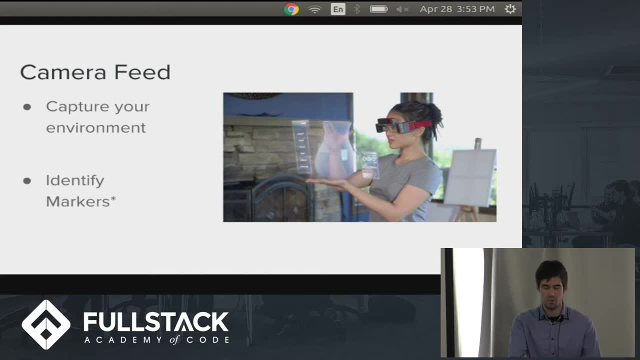 They just appear in your environment and are readily accessible. So now we'll go into kind of the basic requirements for AR. There's four components that you'll need. The first and simplest is just a camera feed. You need this to capture your environment, to identify markers- should maybe be identifiers. 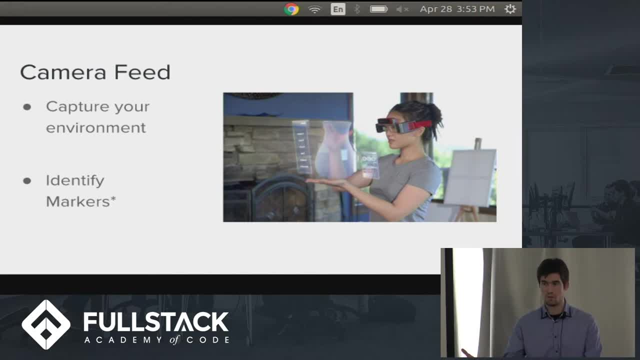 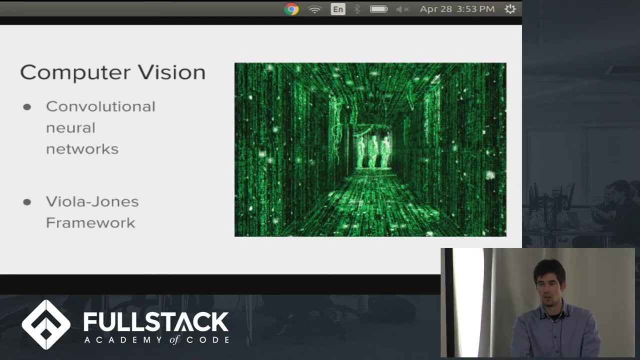 I'll get into why there's an asterisk around that later, For here you can project information. The next step, the next requirement, is definitely the most important, the most difficult. It's kind of the magic of AR happens here, and it's through computer vision. This field deals. 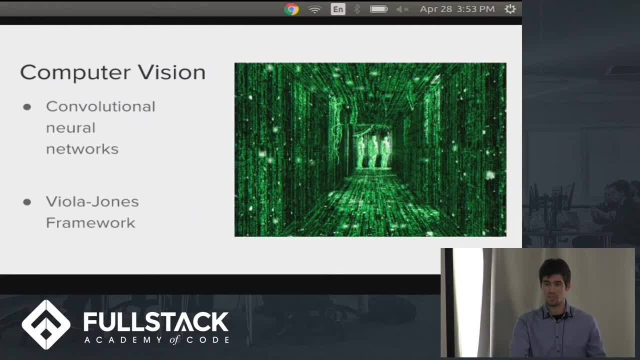 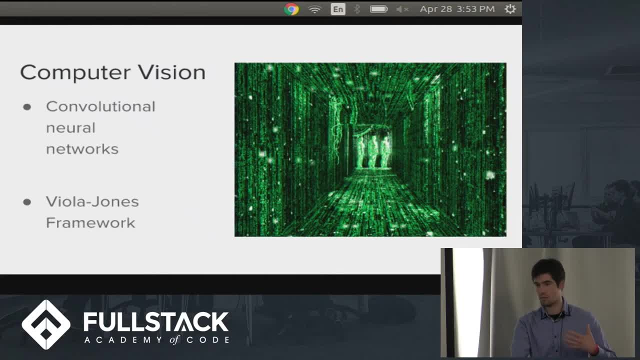 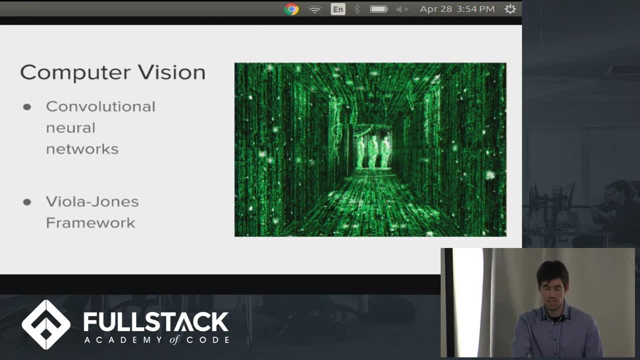 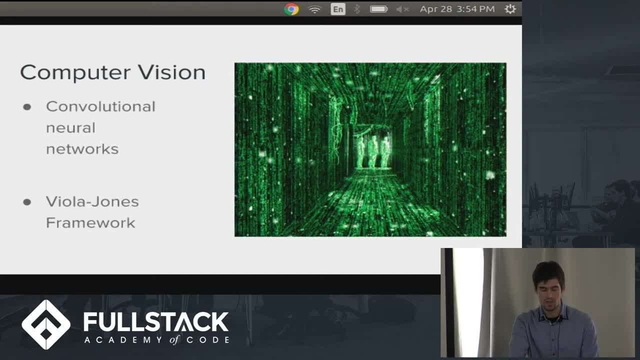 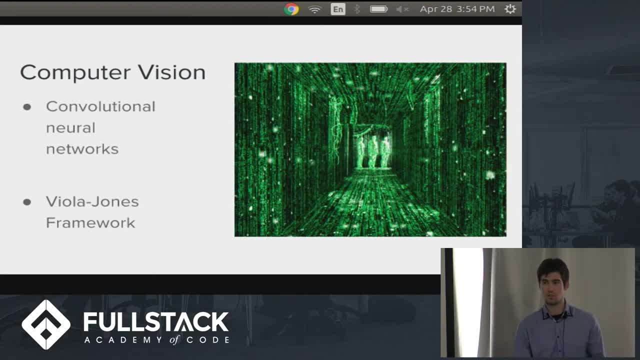 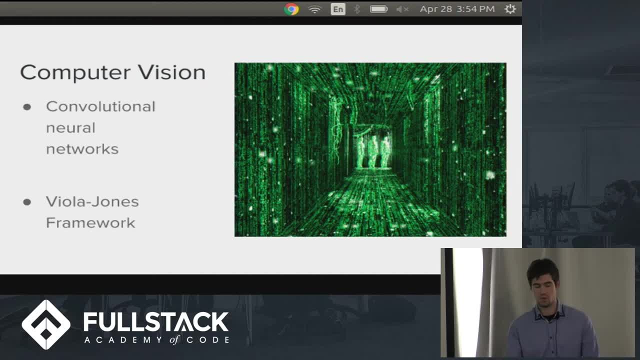 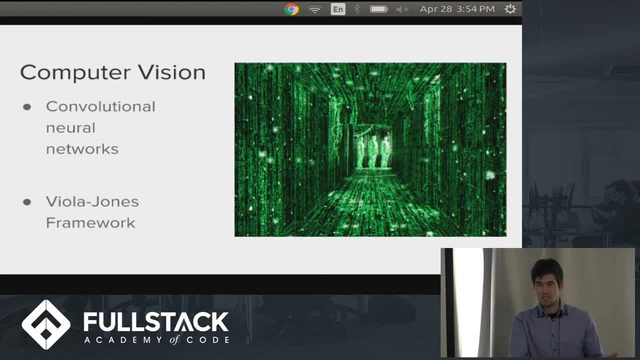 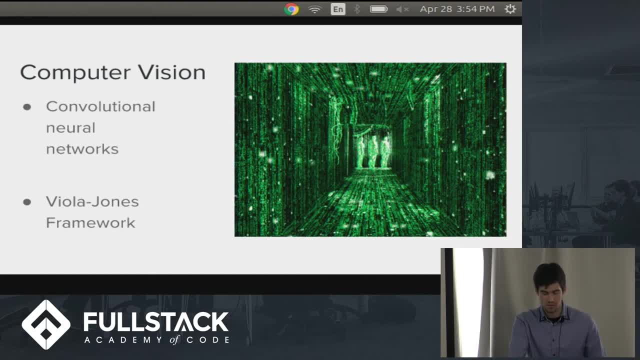 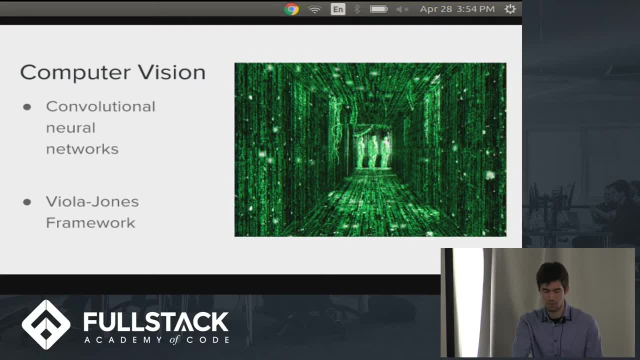 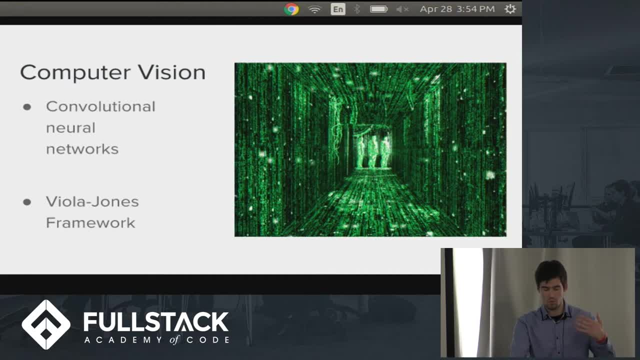 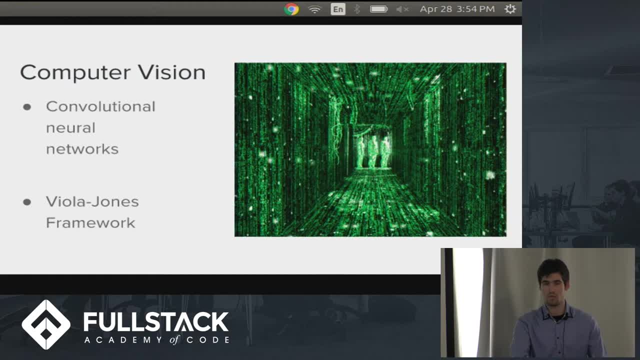 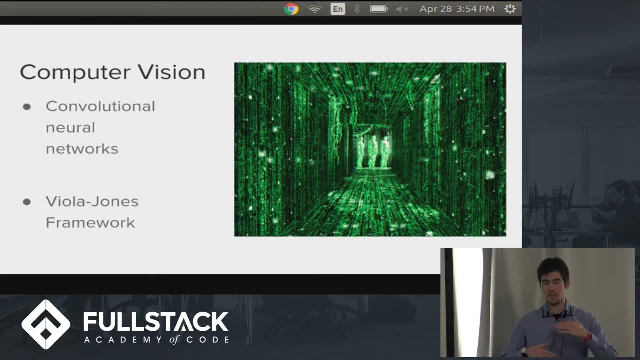 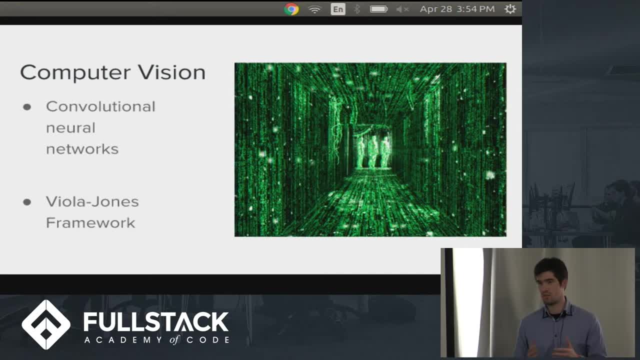 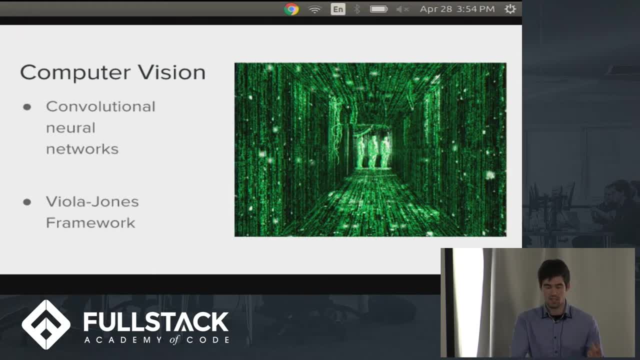 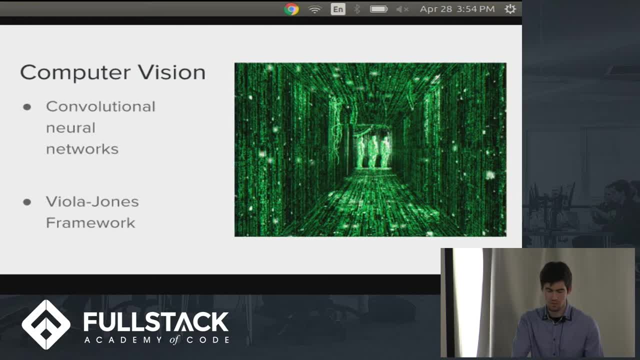 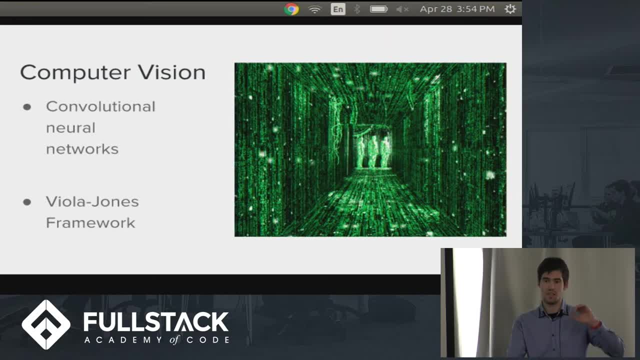 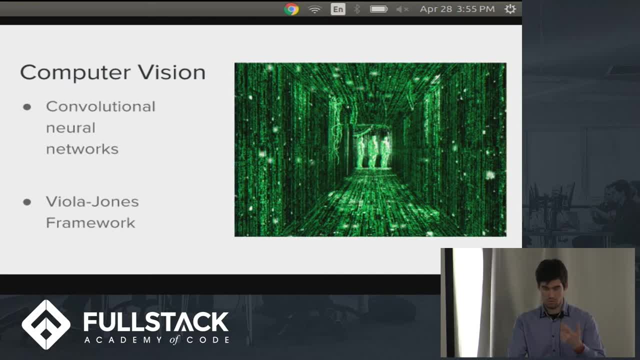 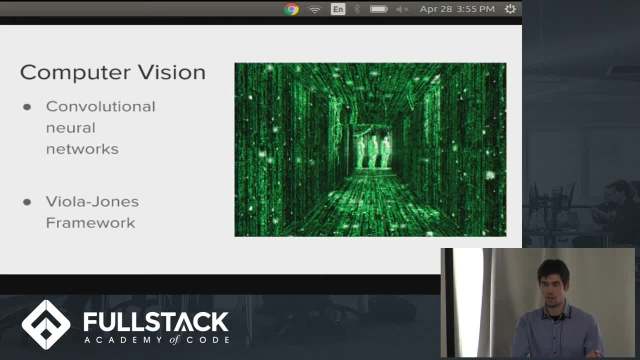 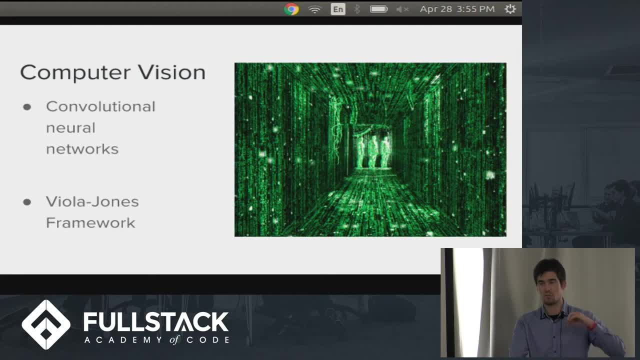 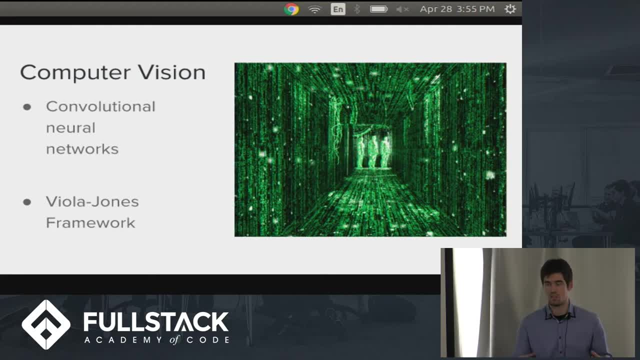 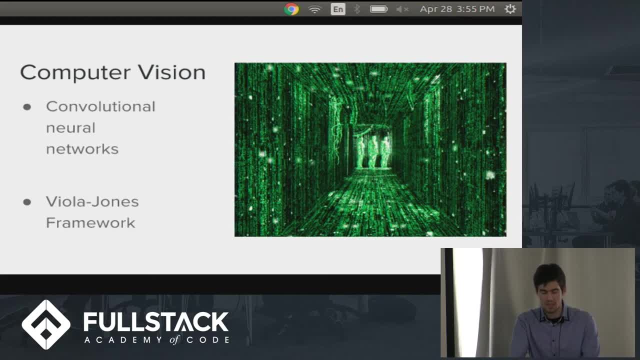 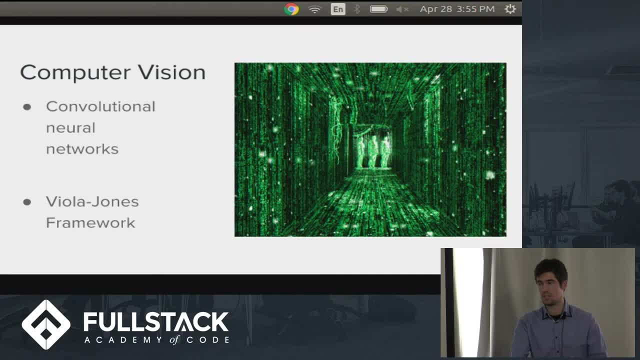 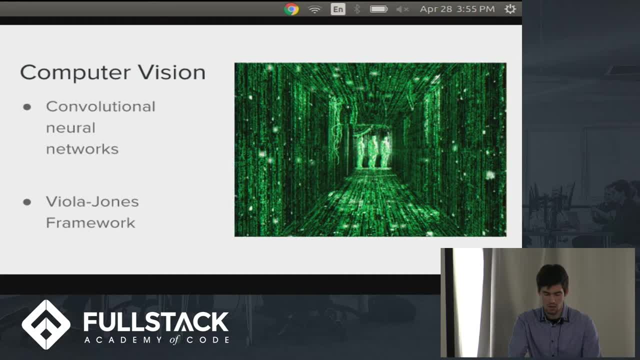 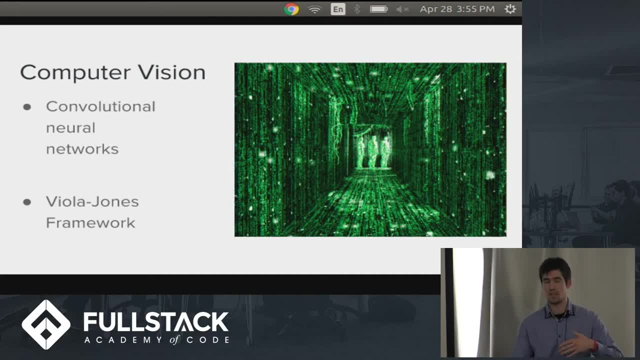 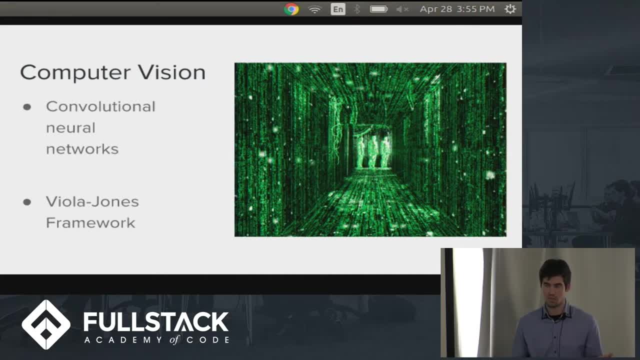 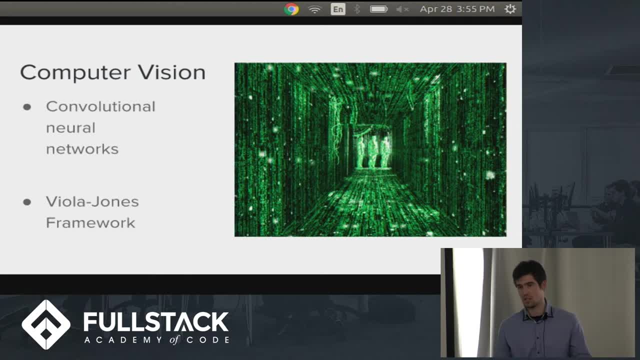 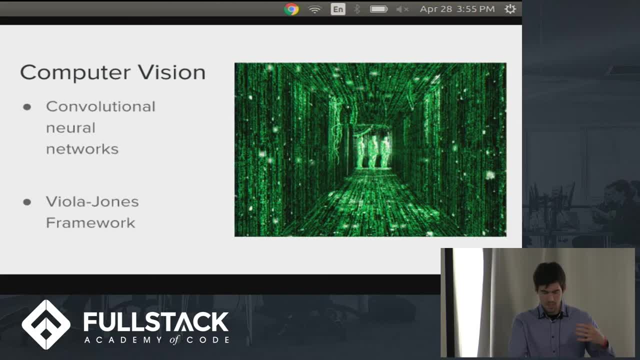 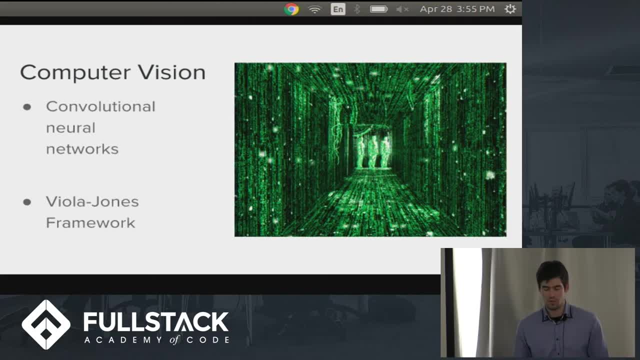 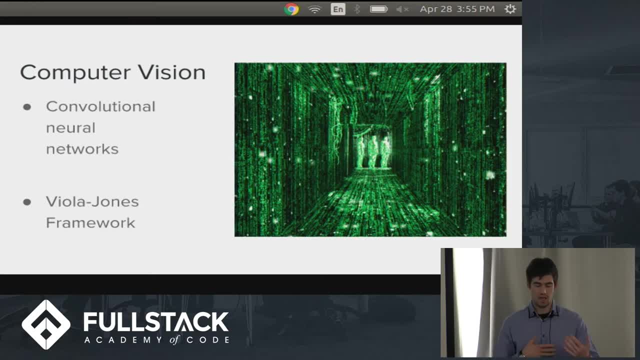 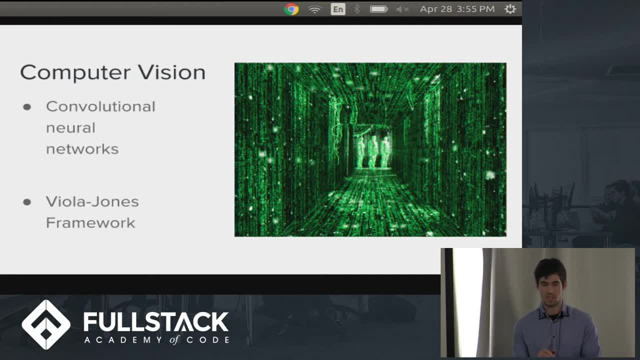 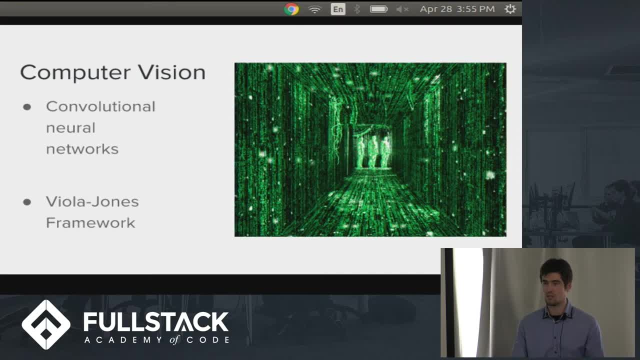 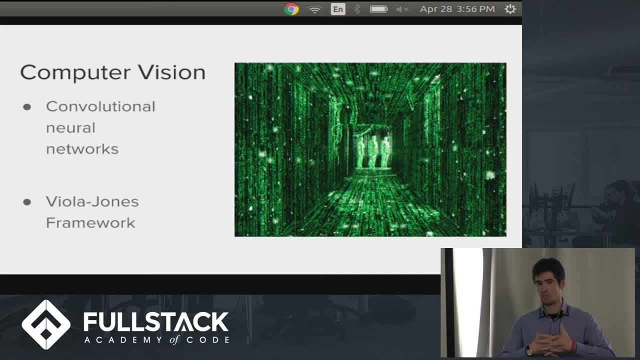 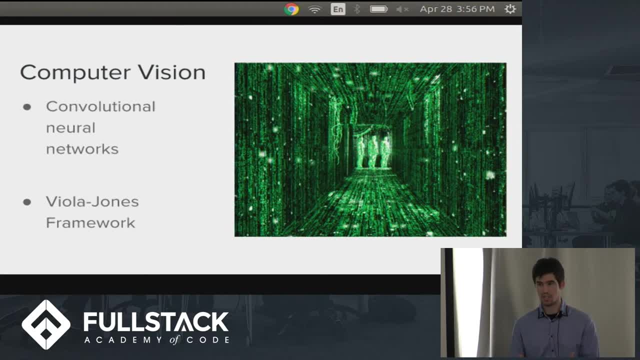 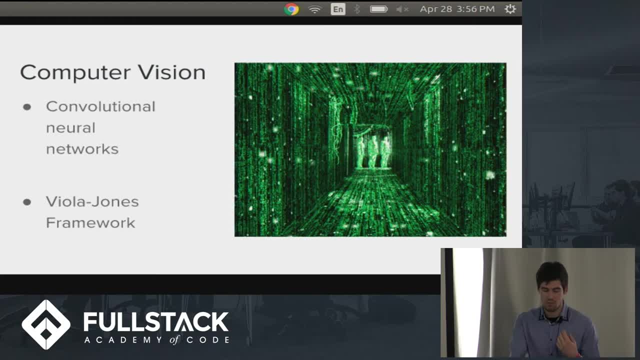 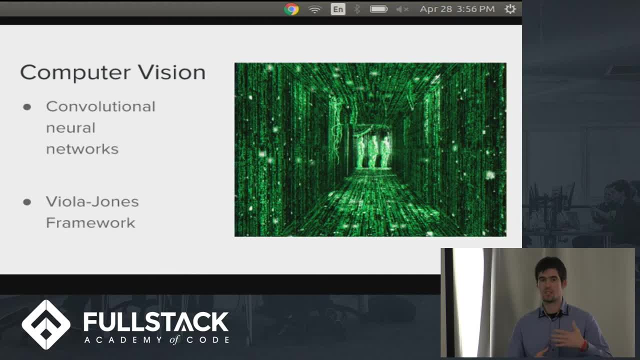 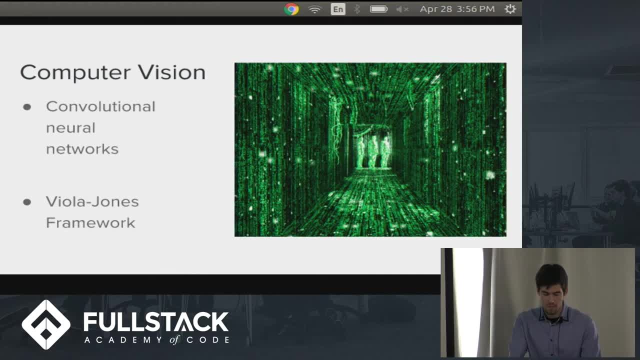 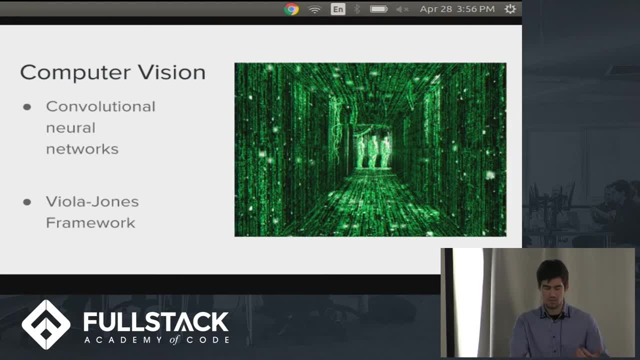 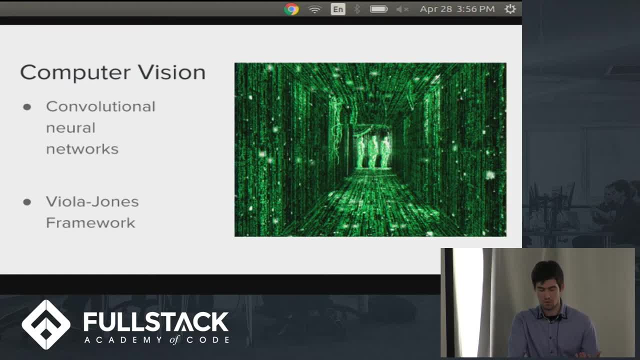 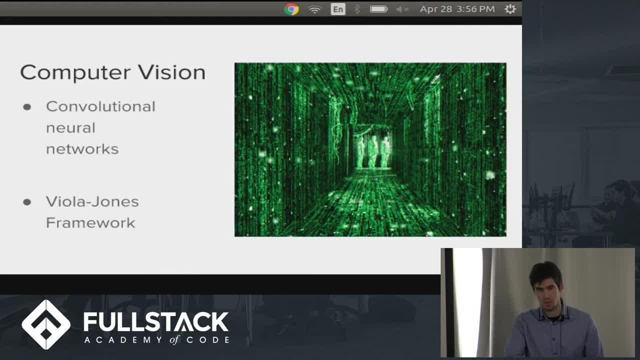 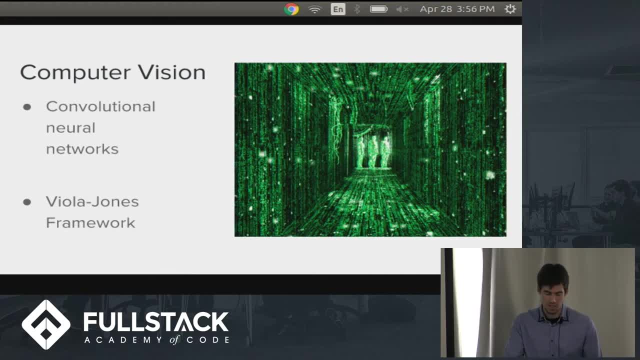 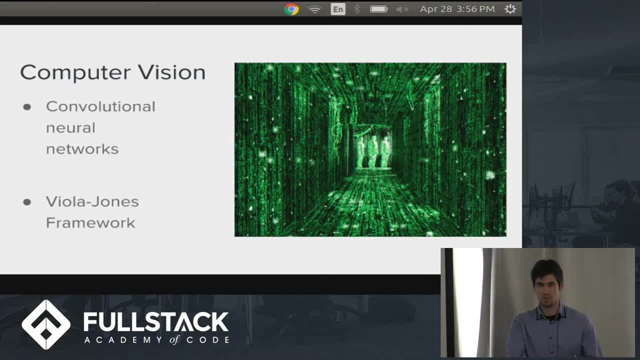 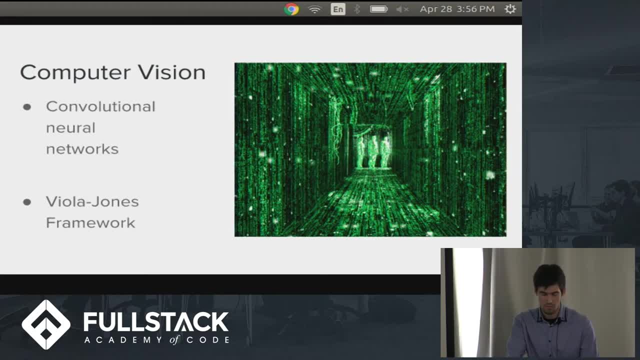 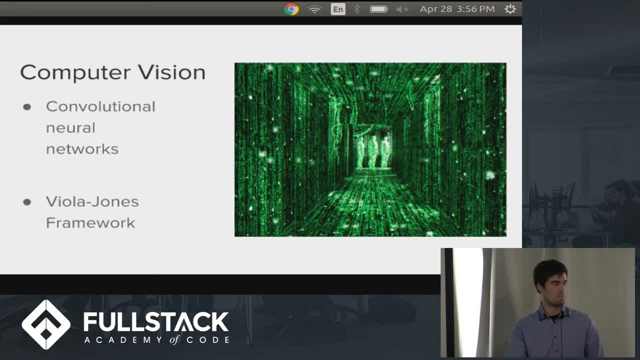 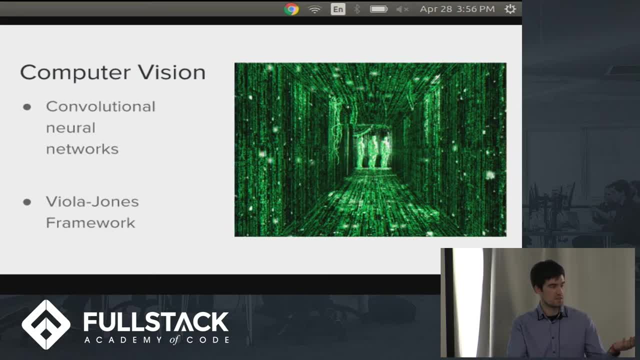 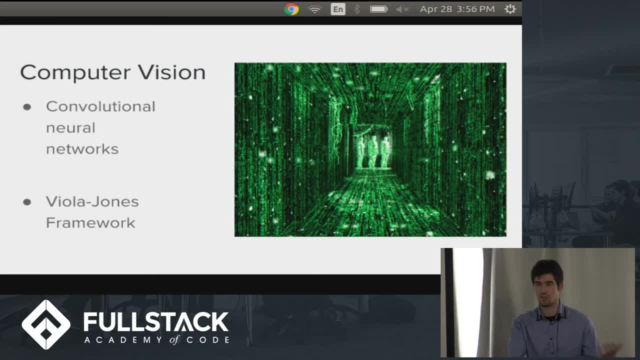 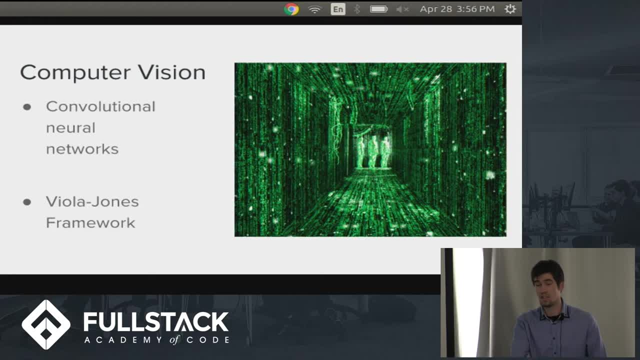 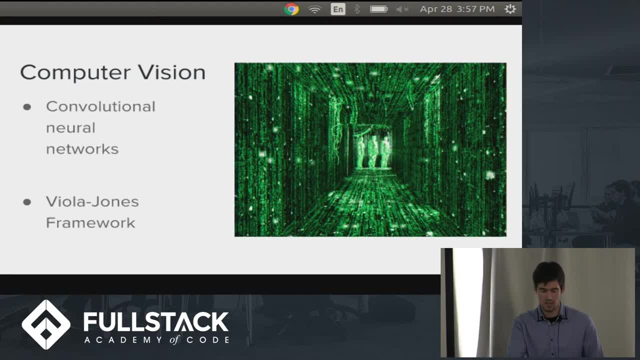 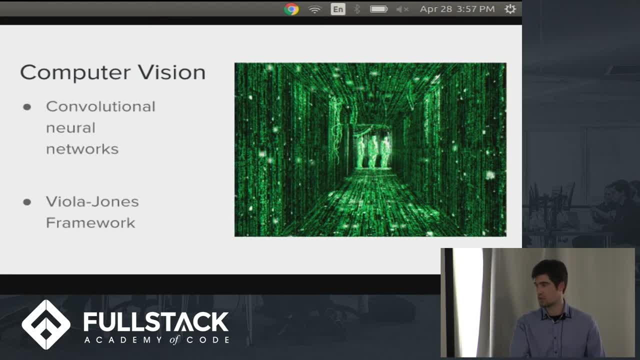 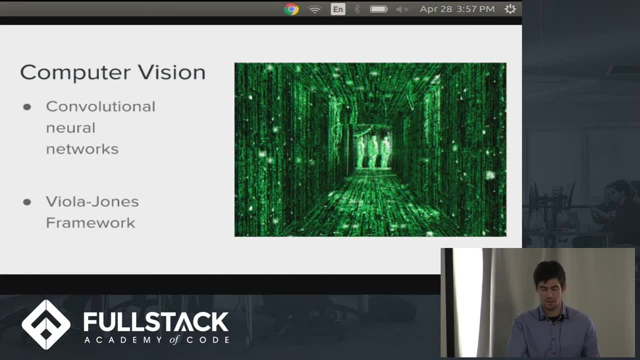 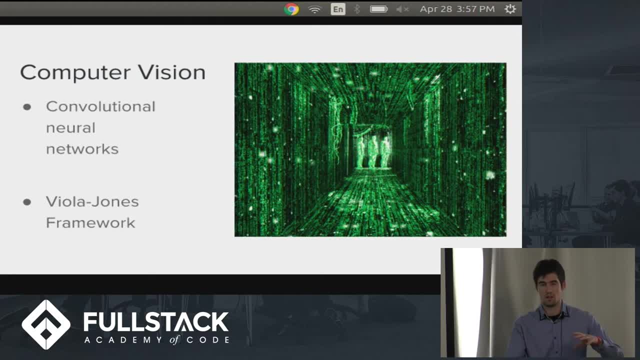 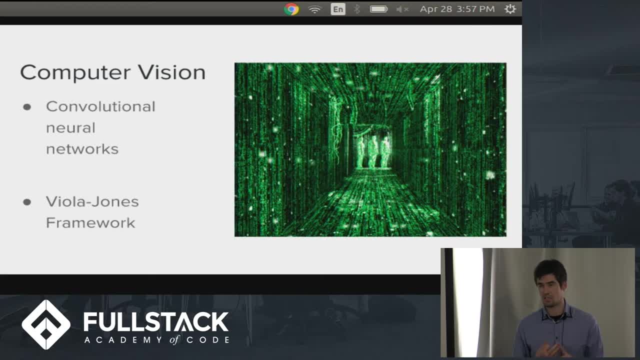 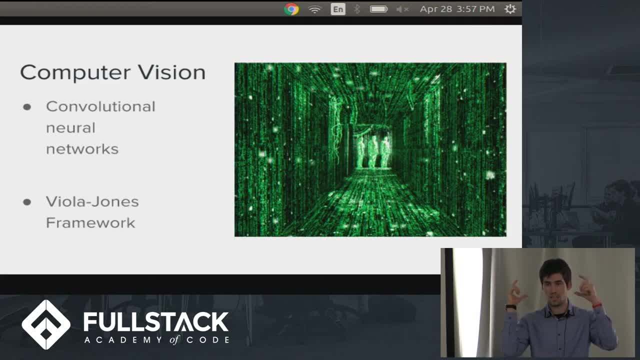 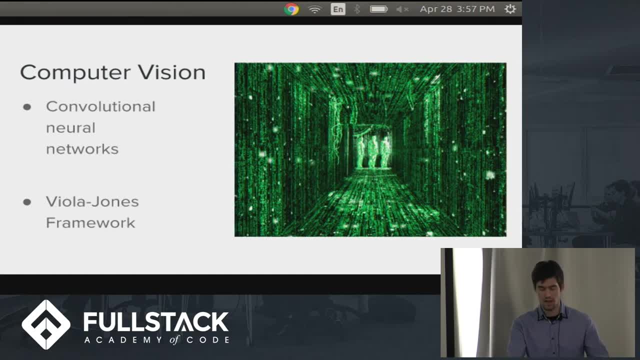 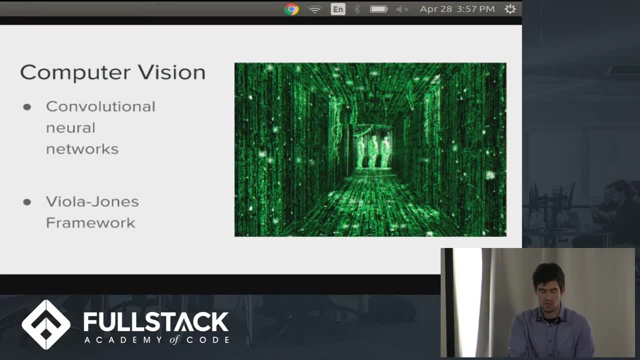 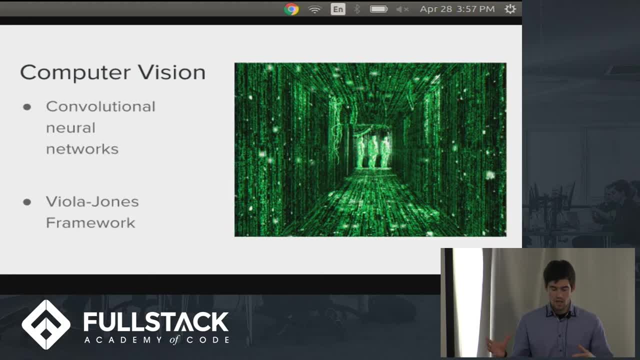 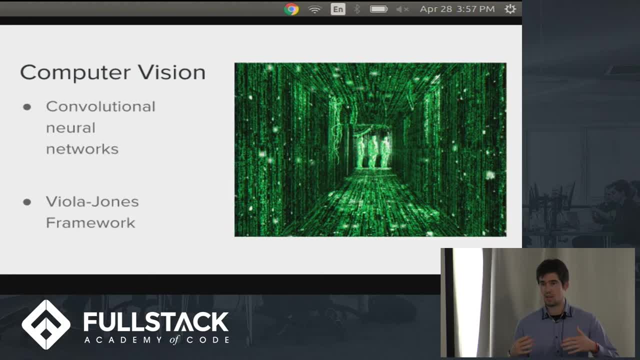 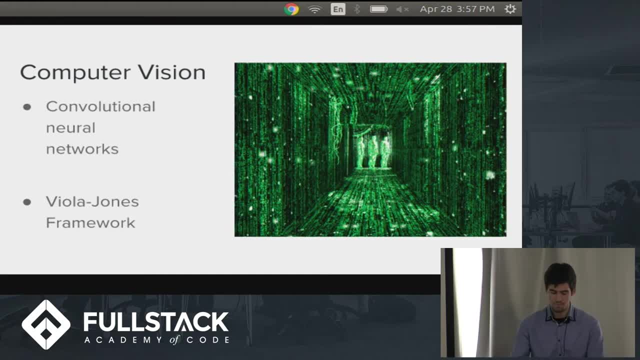 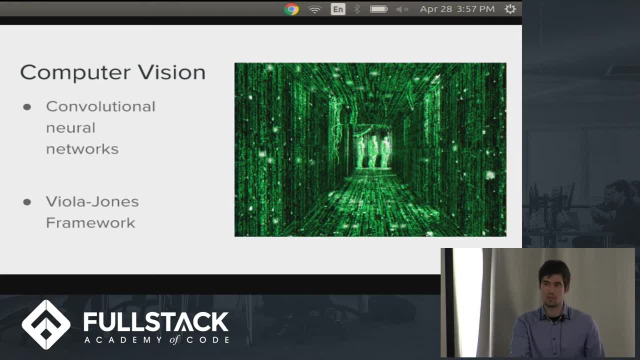 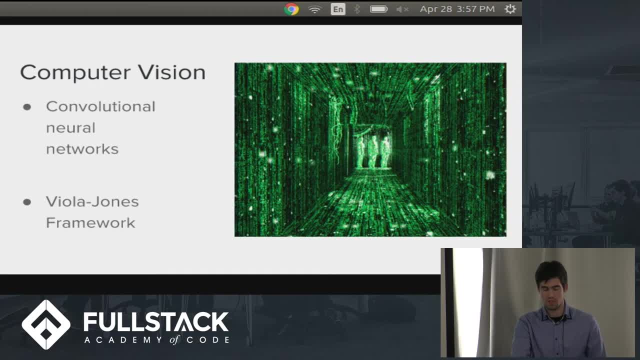 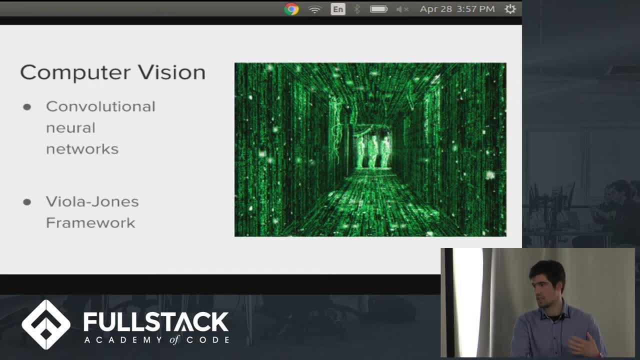 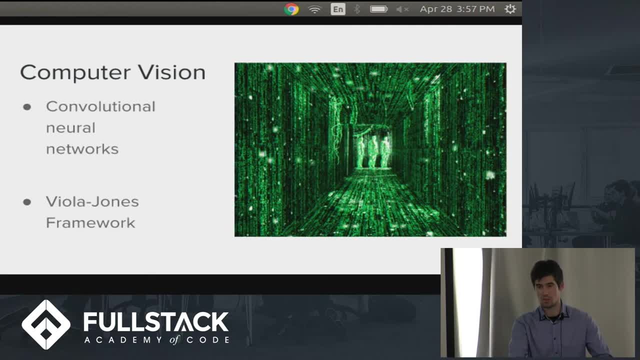 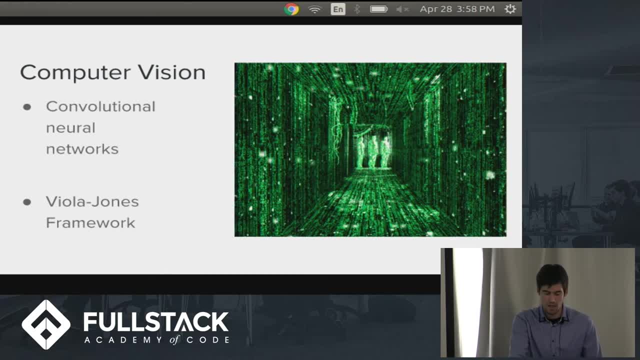 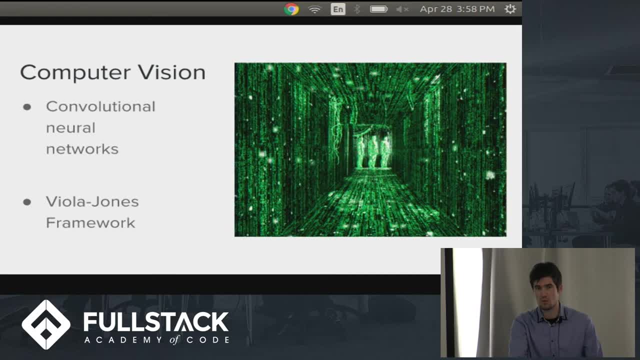 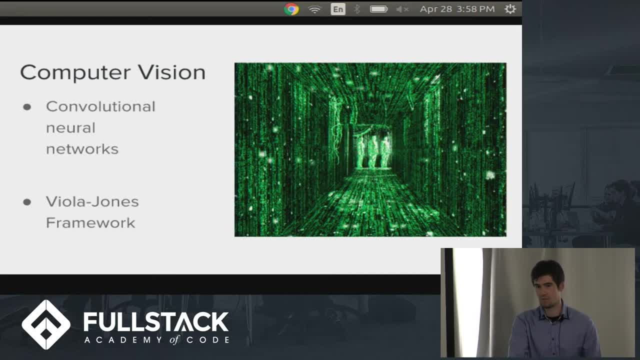 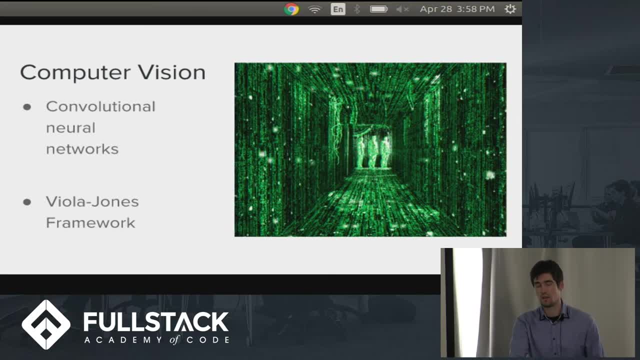 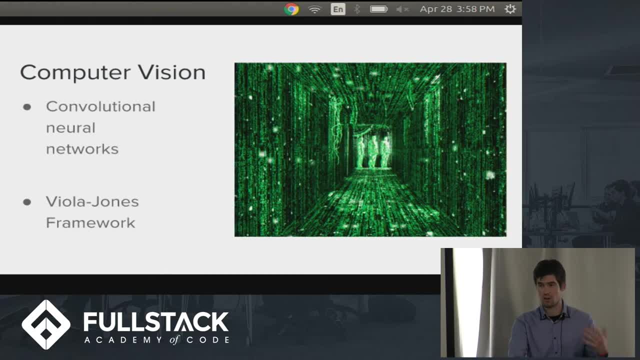 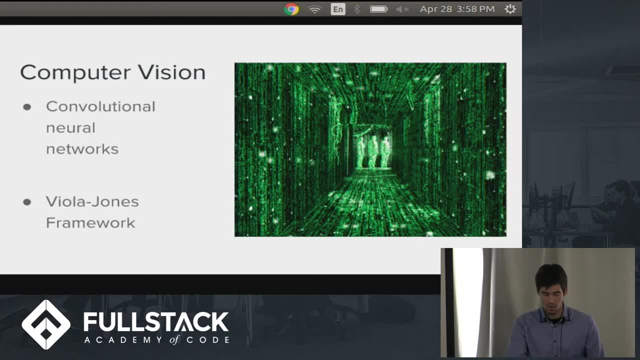 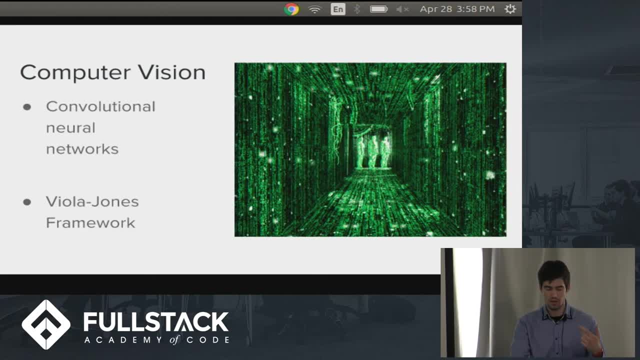 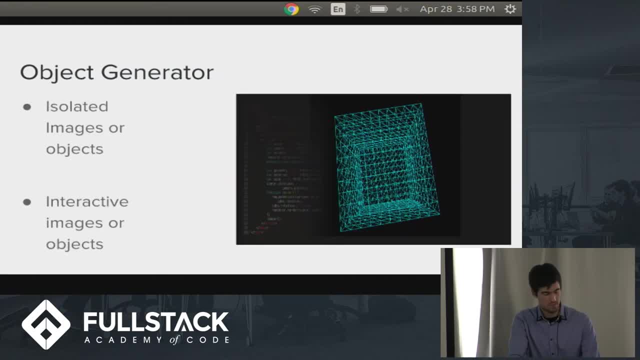 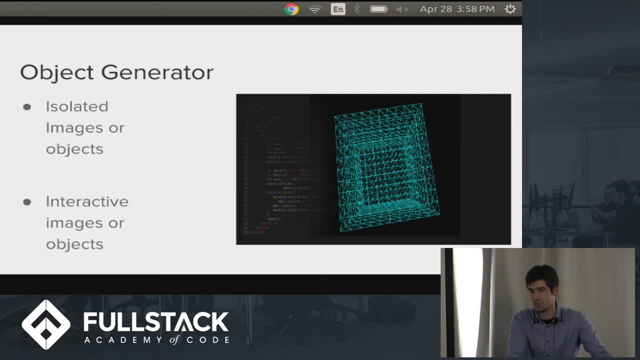 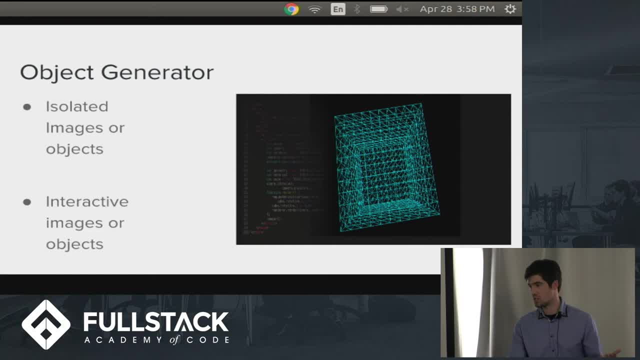 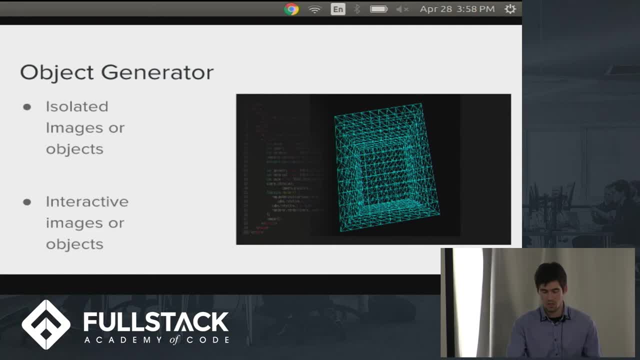 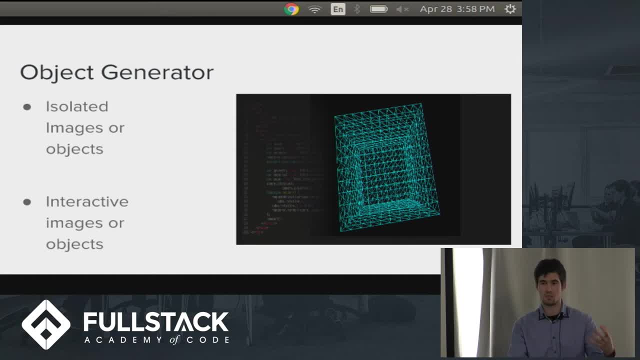 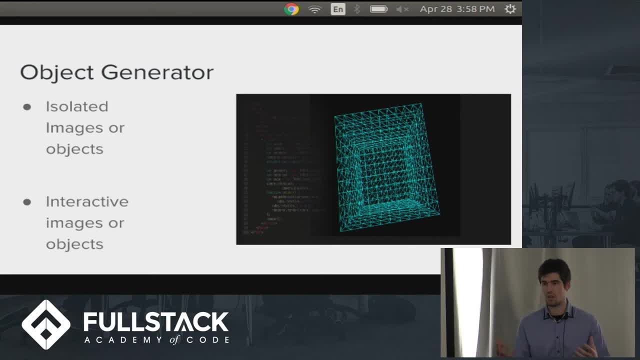 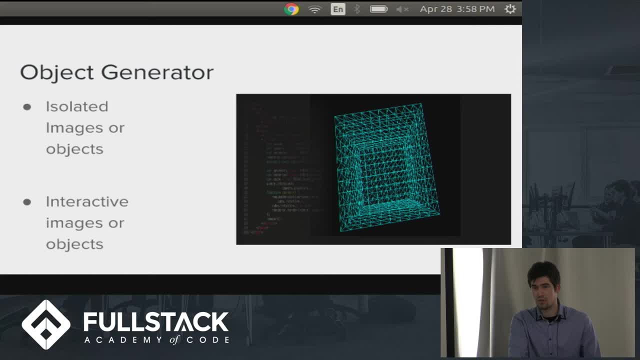 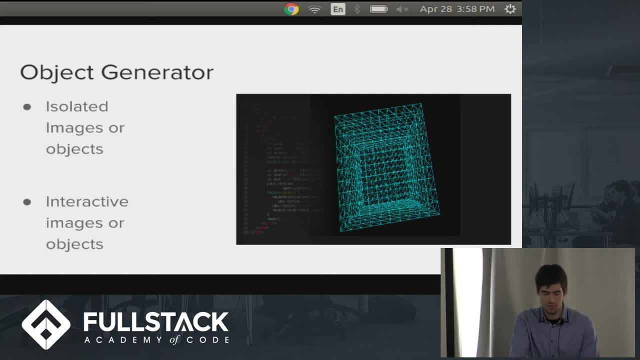 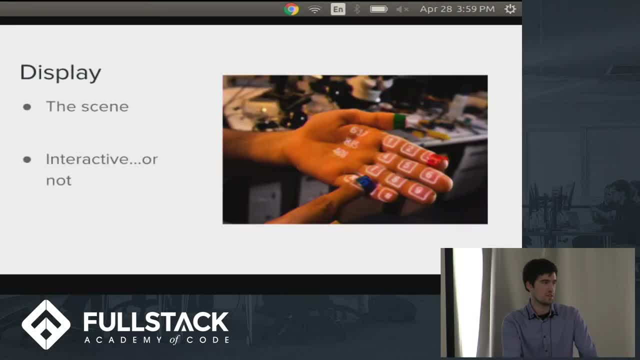 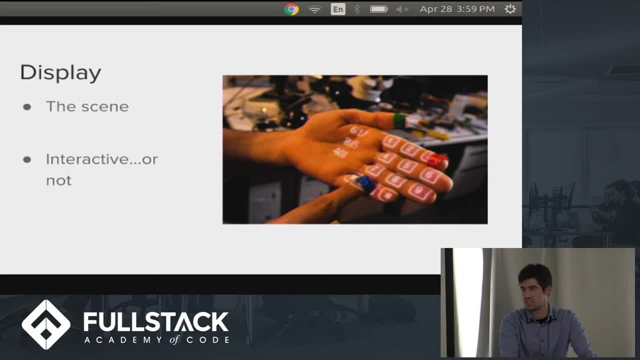 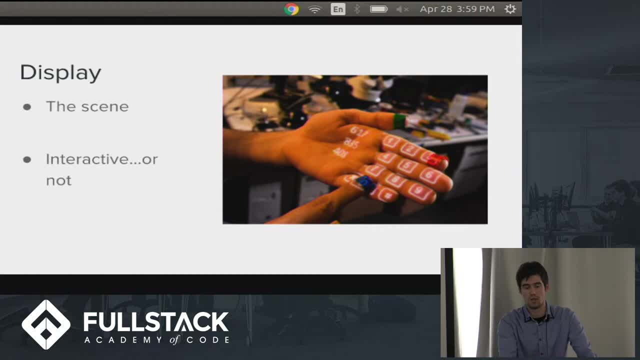 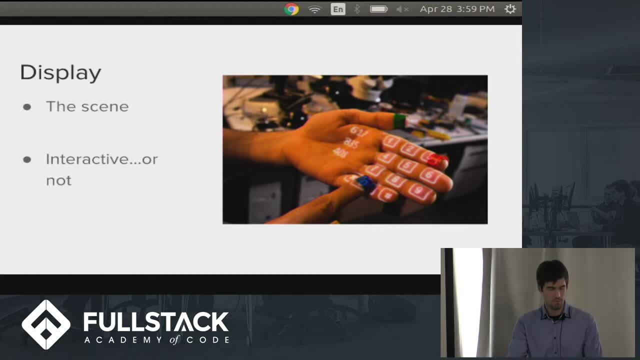 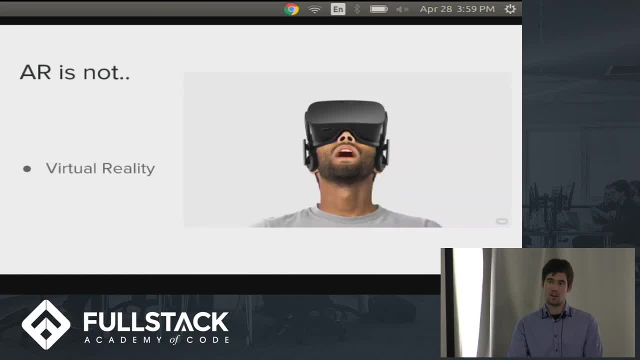 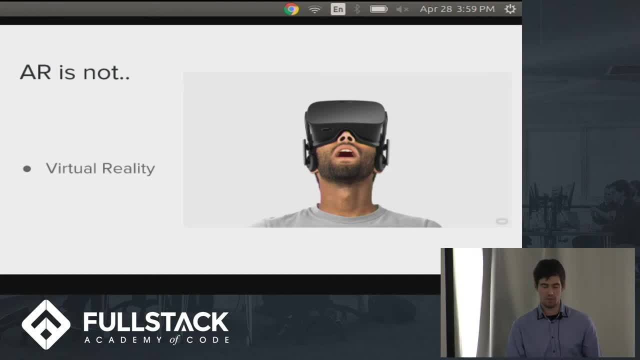 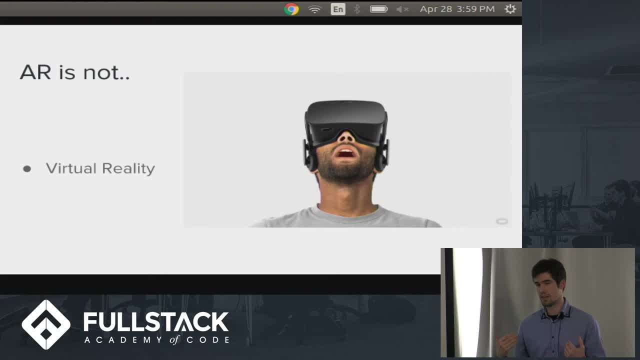 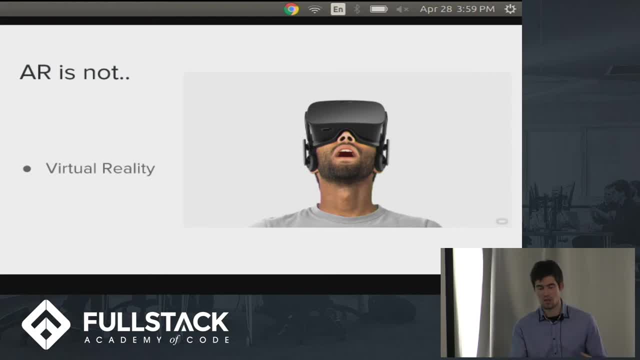 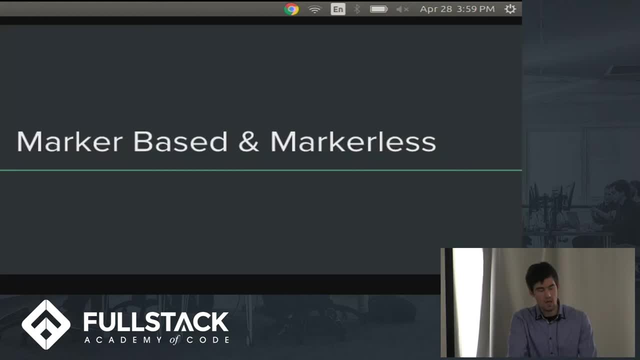 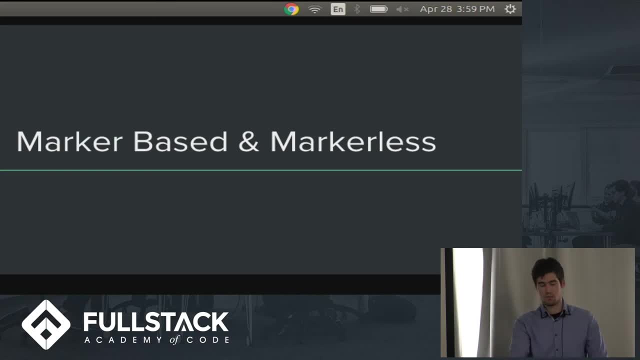 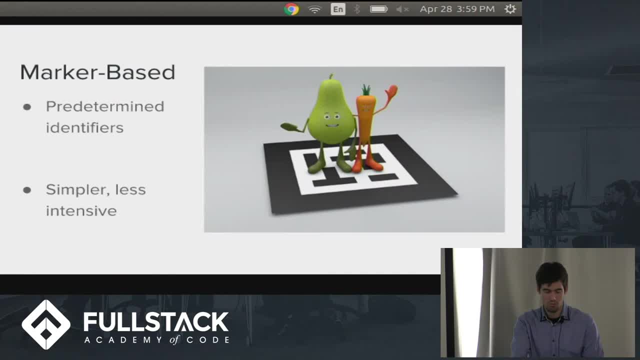 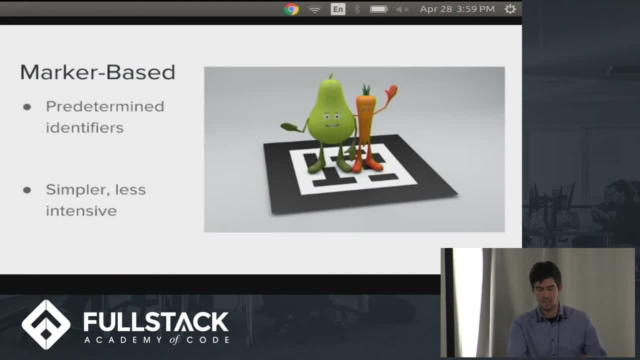 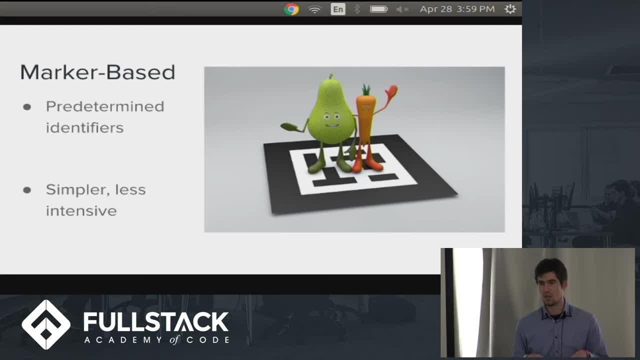 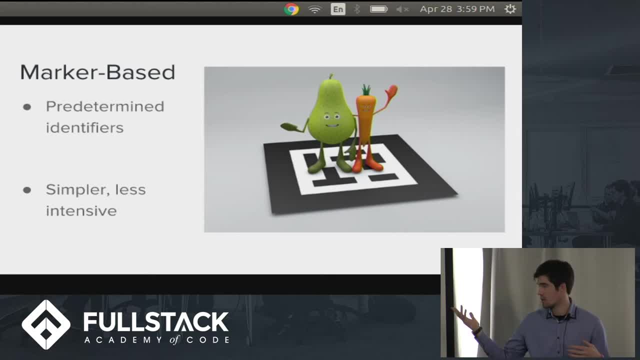 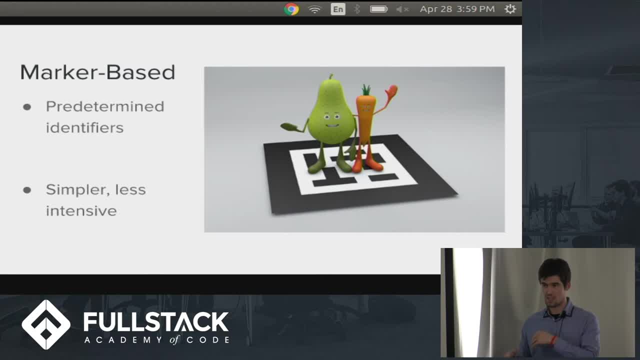 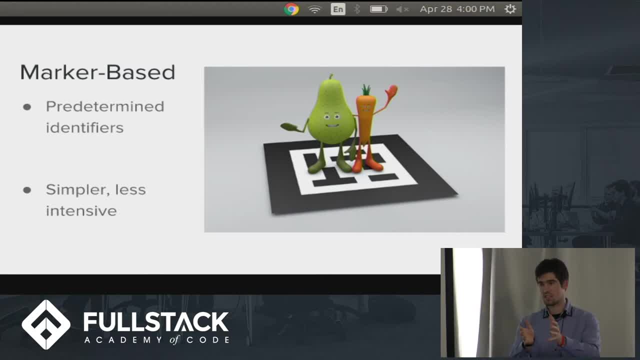 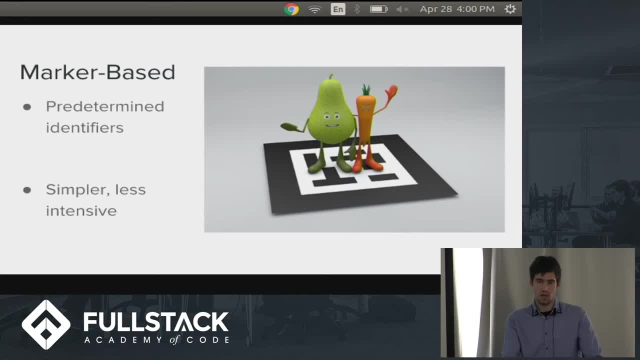 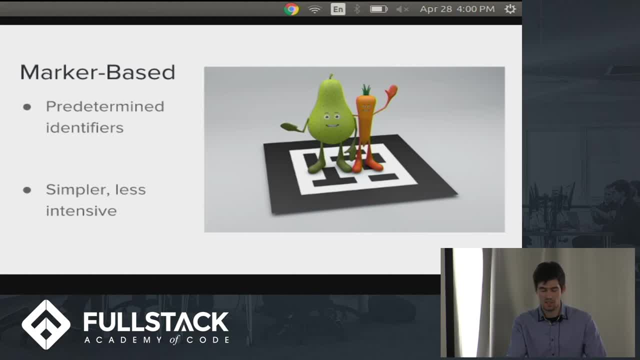 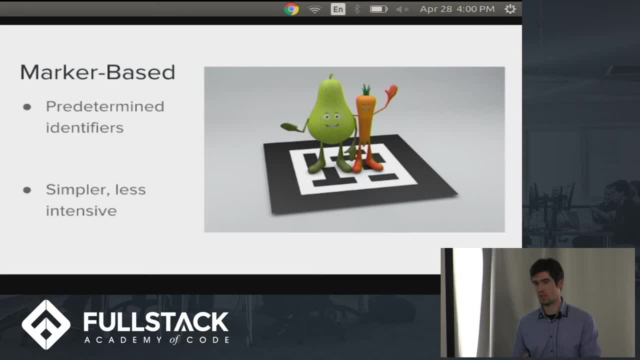 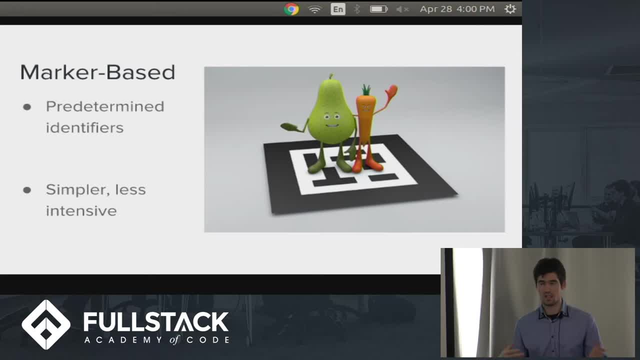 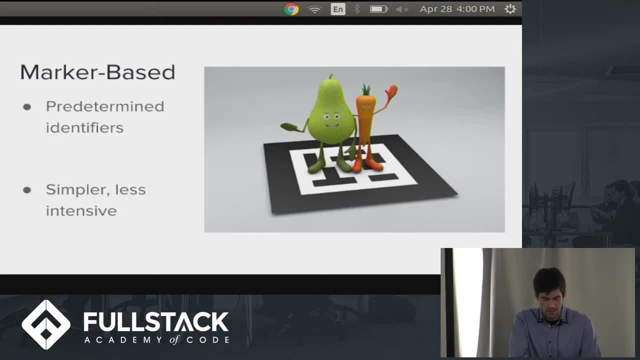 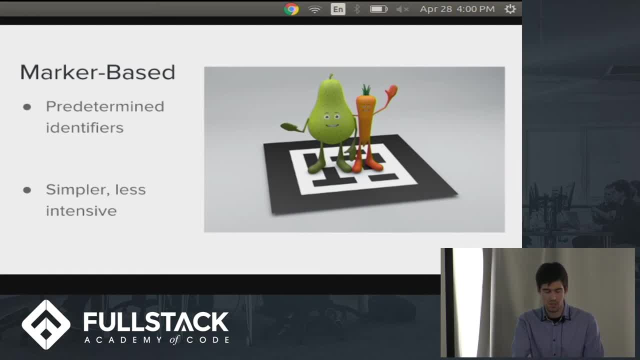 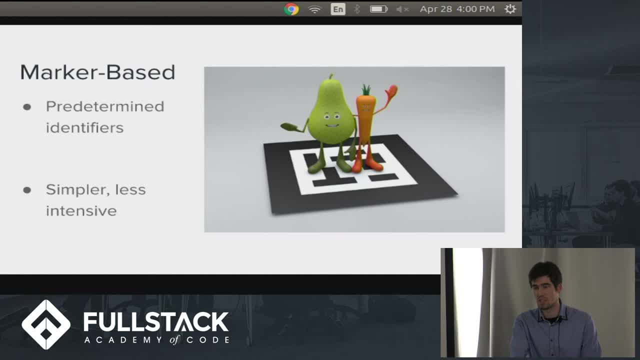 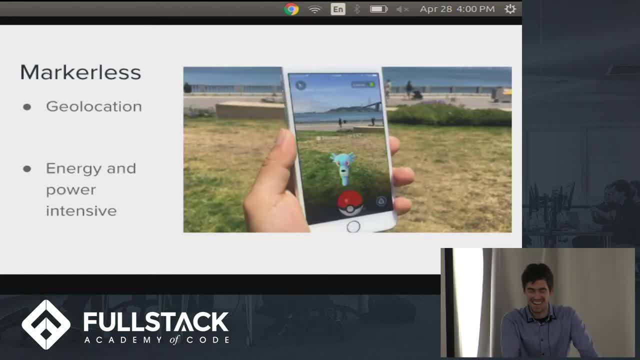 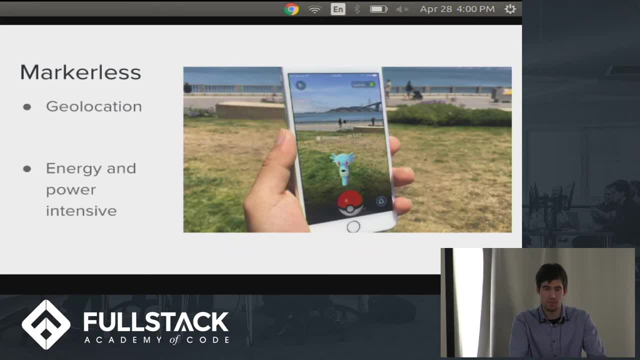 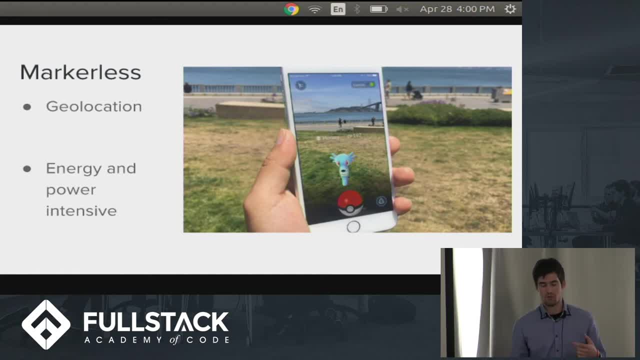 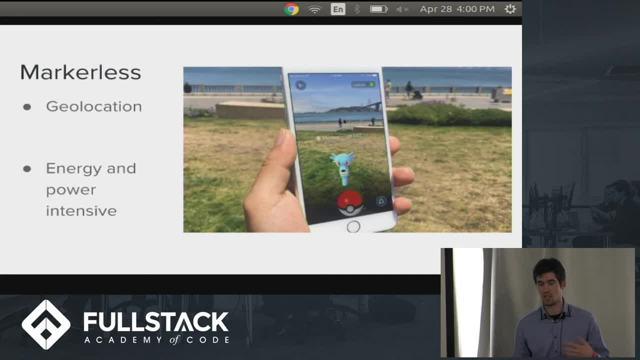 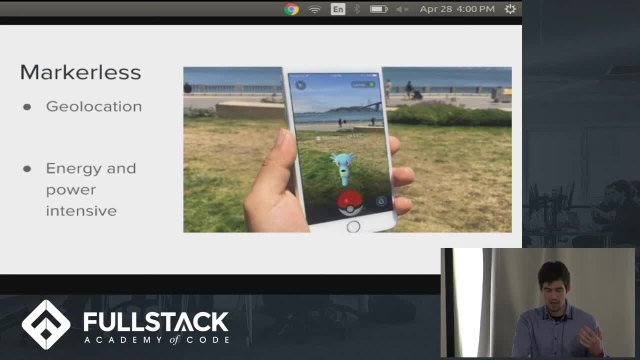 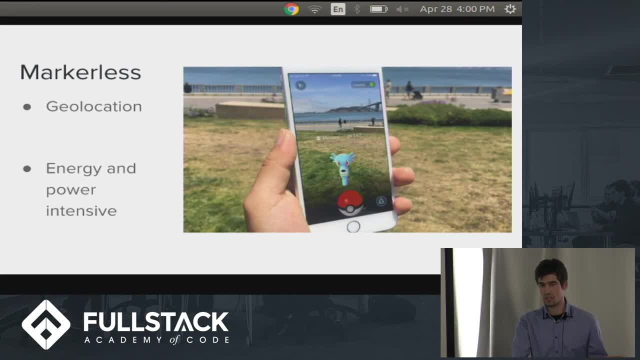 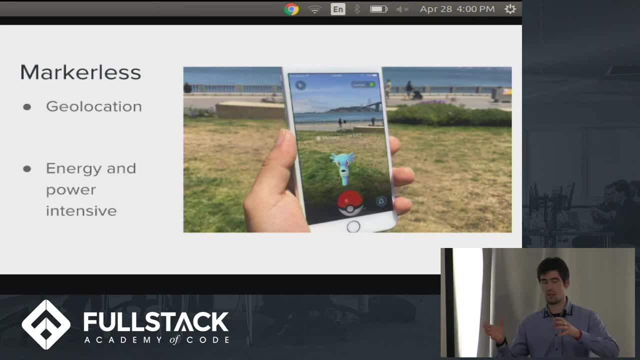 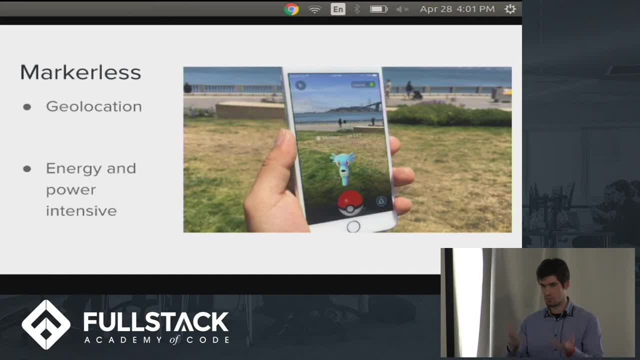 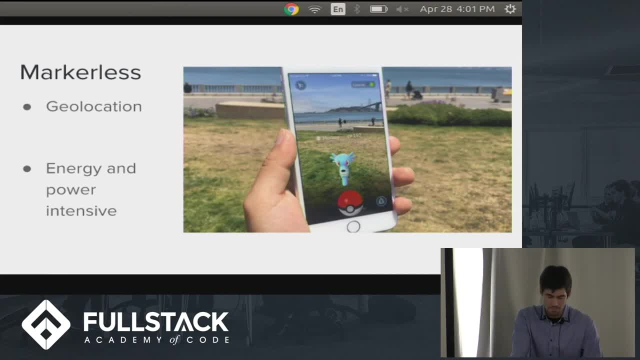 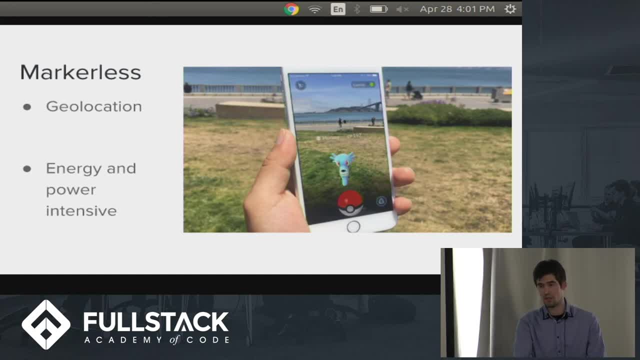 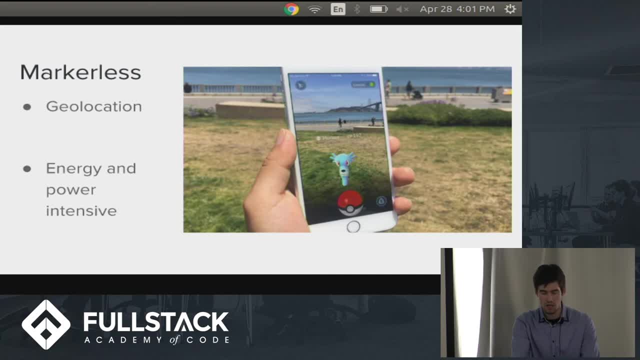 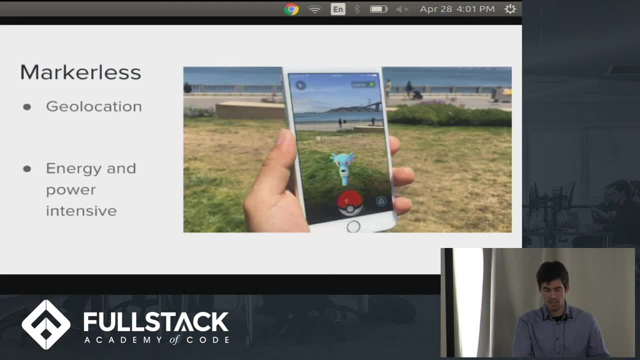 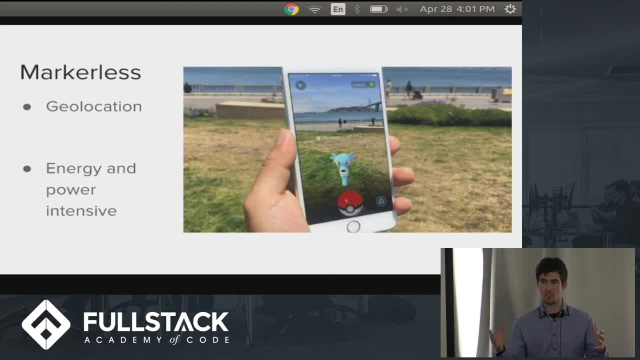 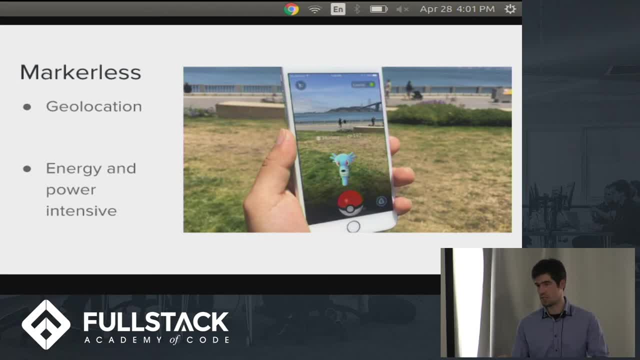 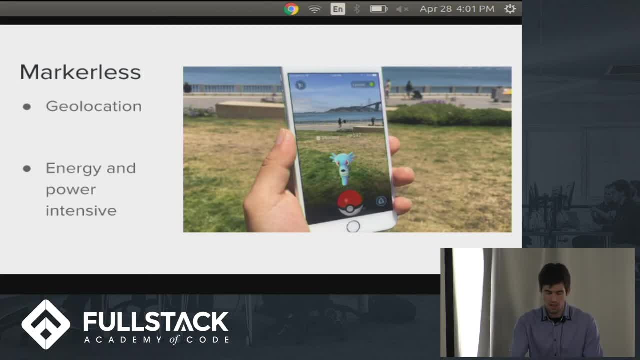 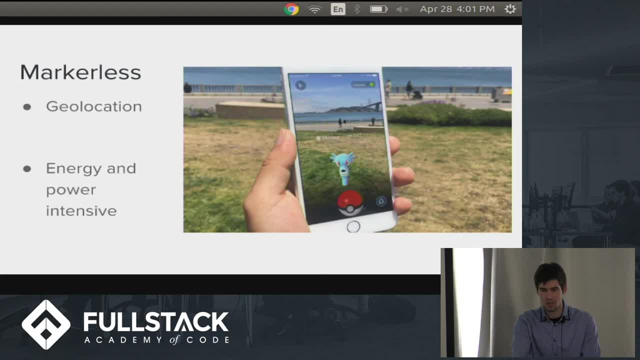 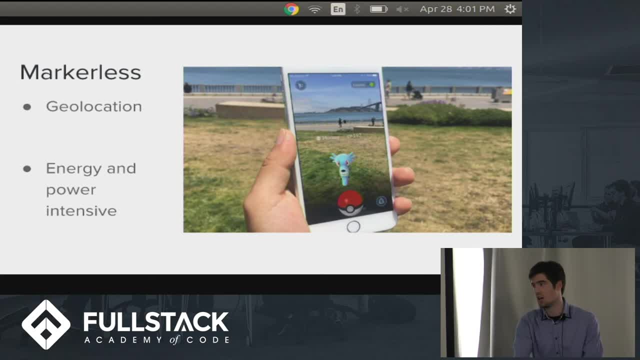 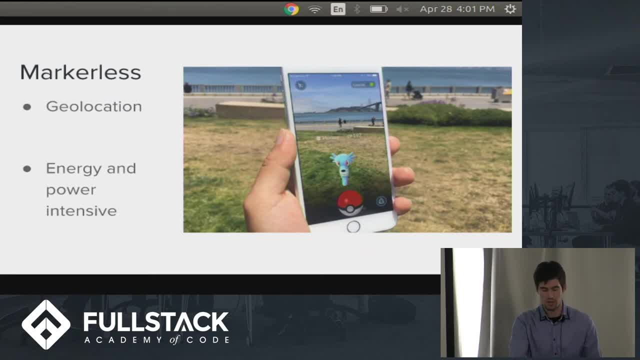 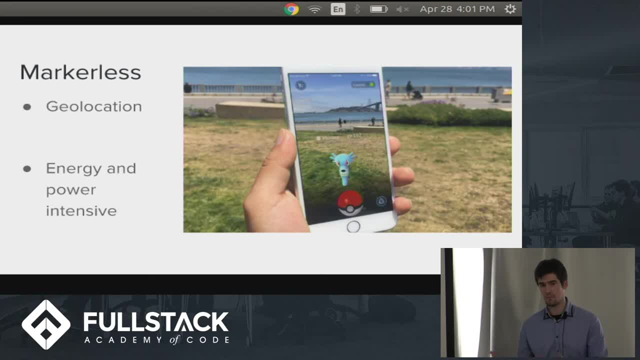 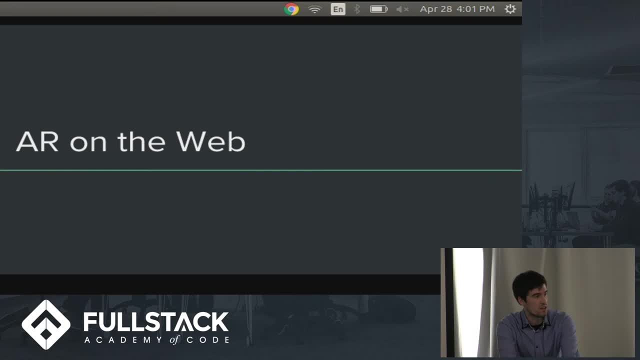 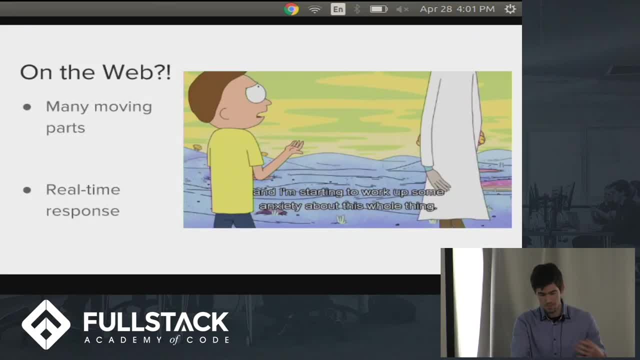 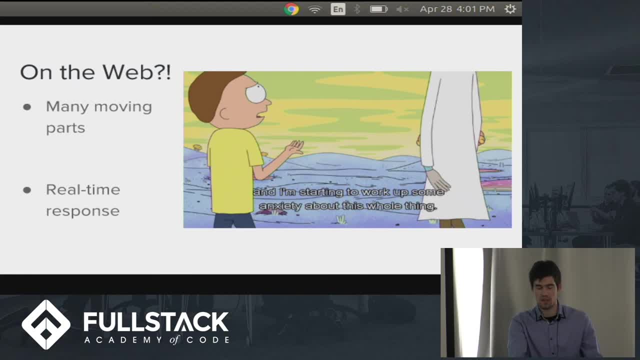 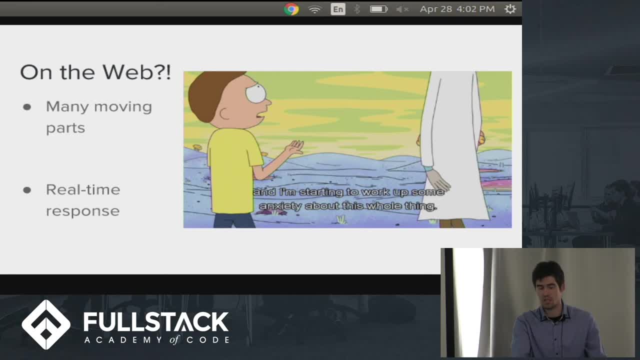 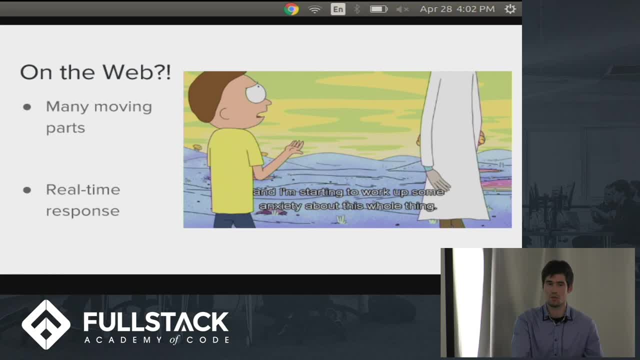 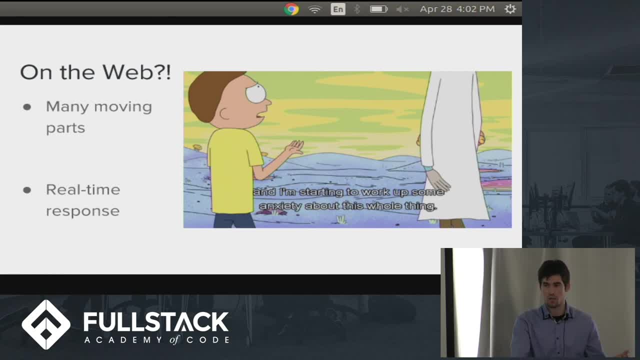 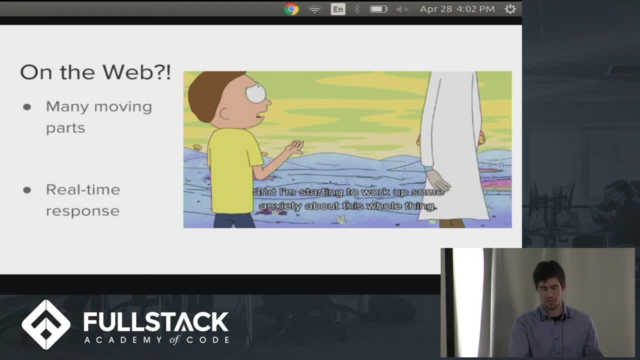 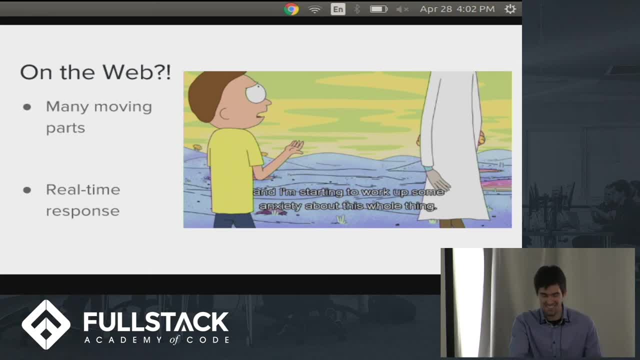 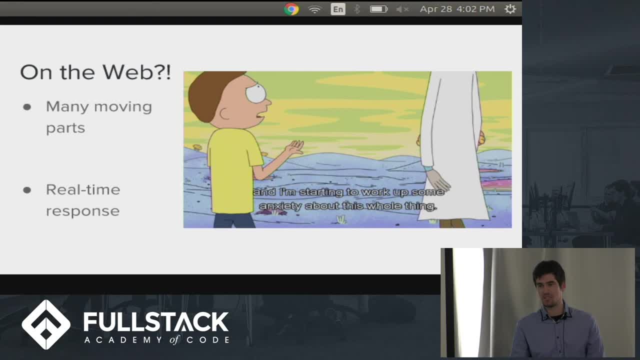 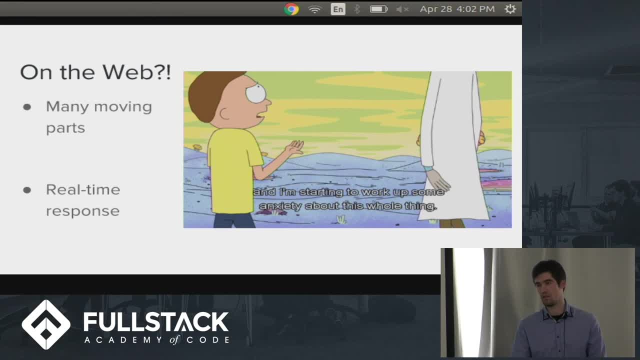 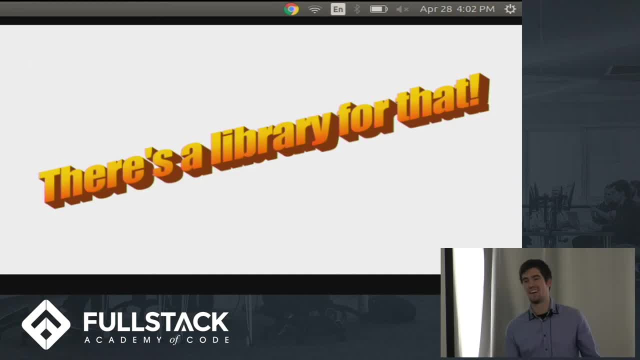 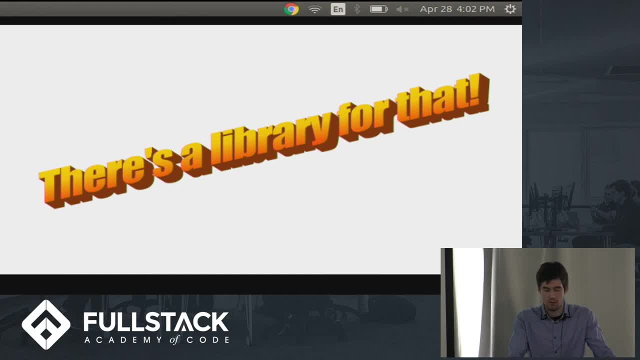 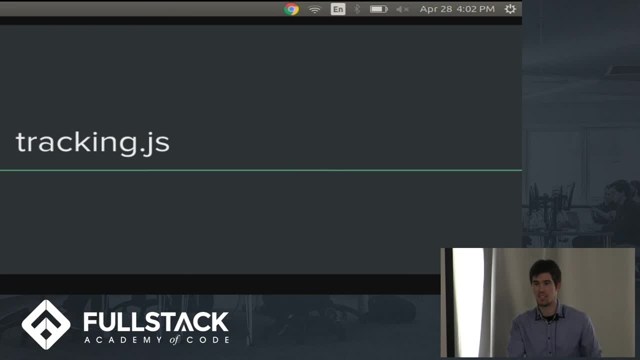 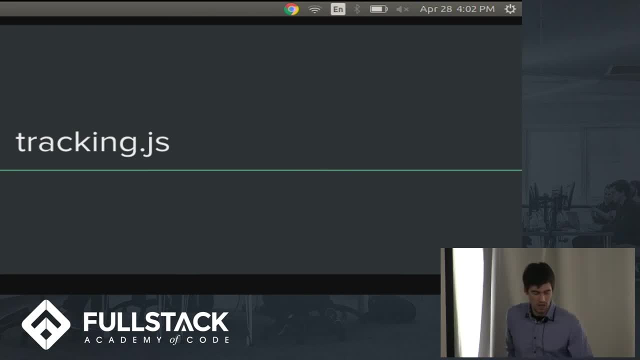 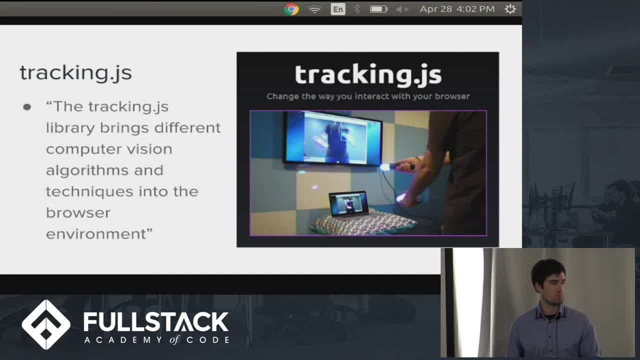 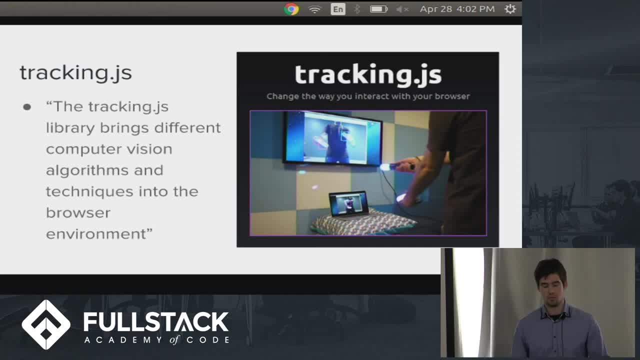 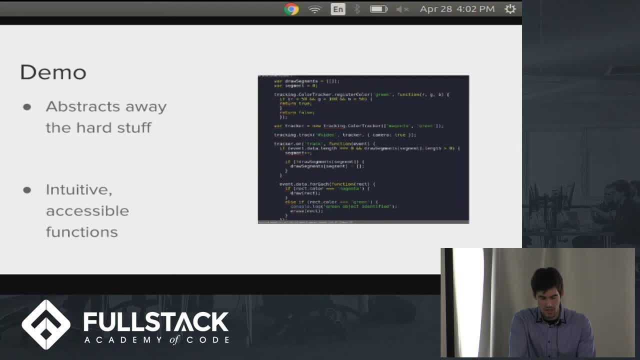 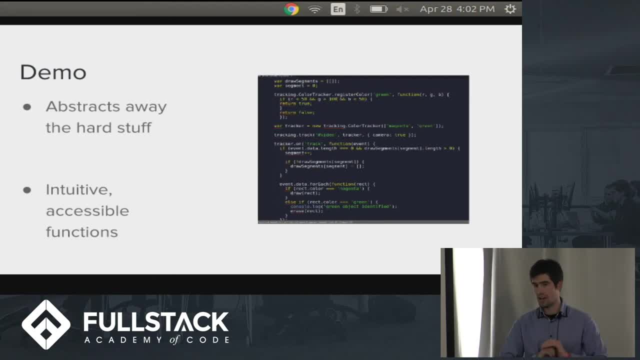 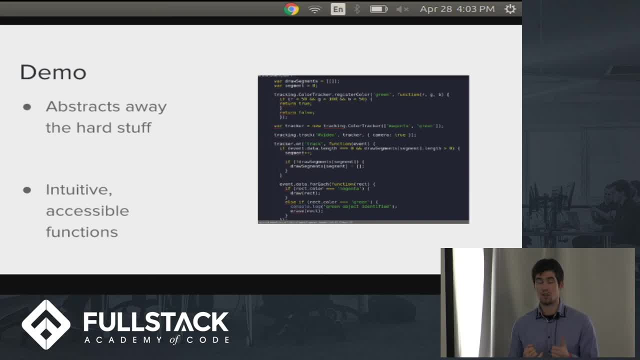 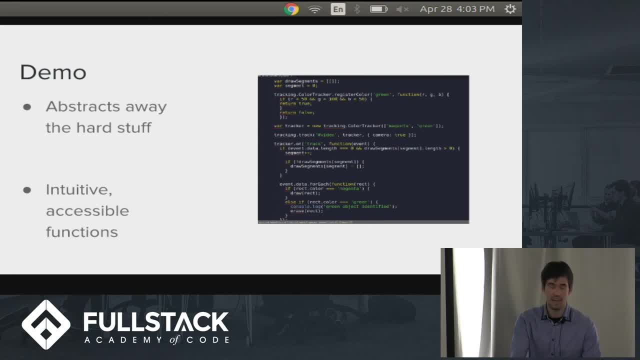 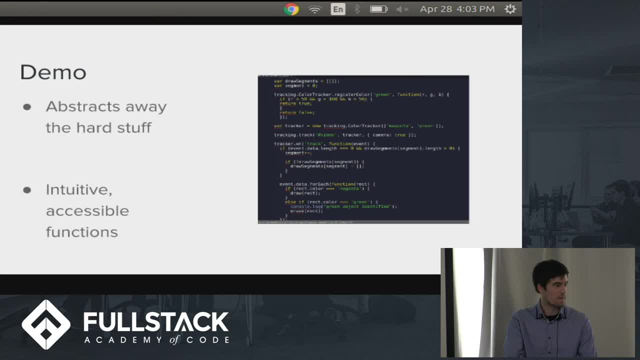 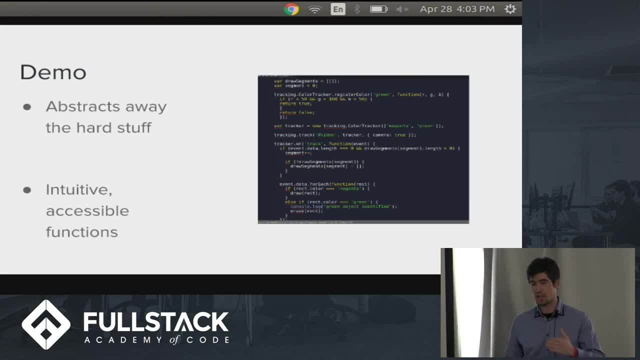 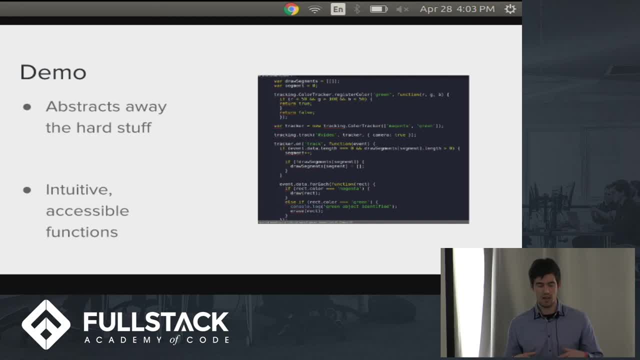 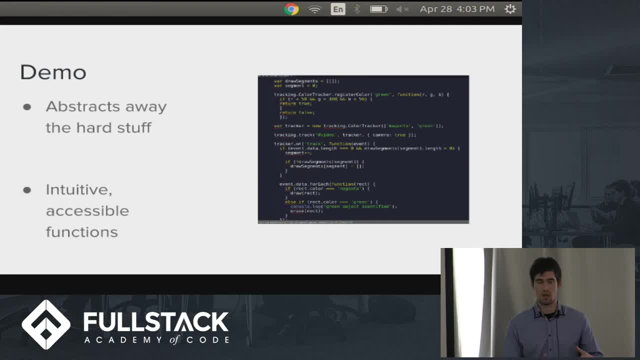 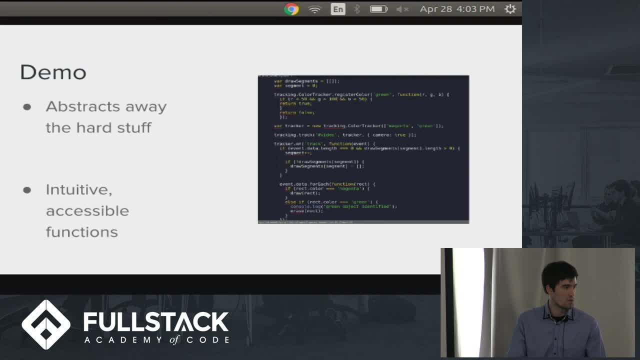 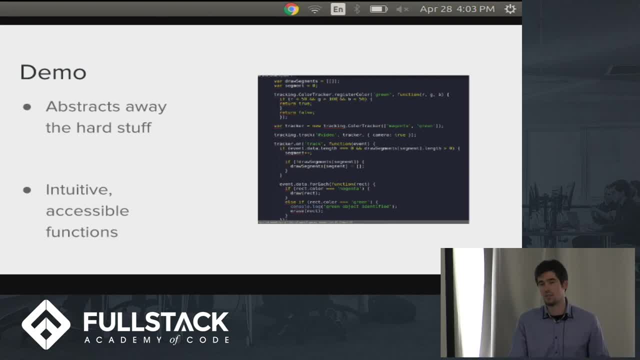 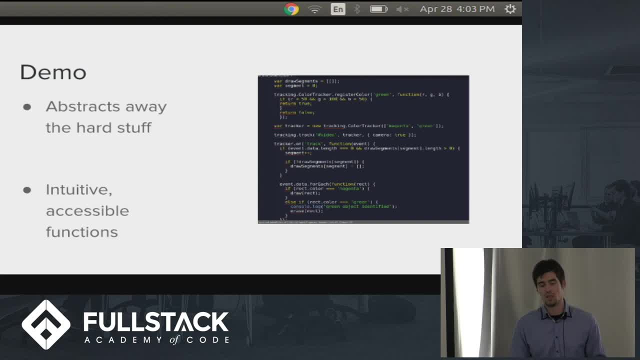 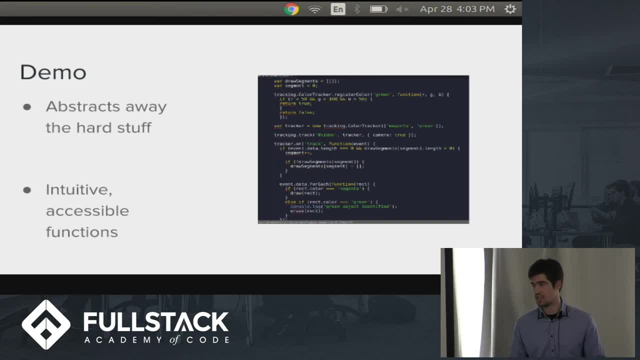 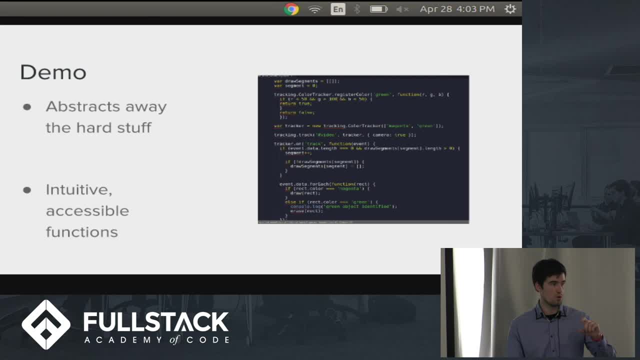 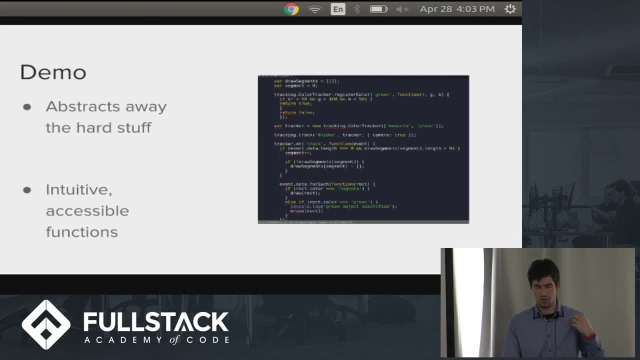 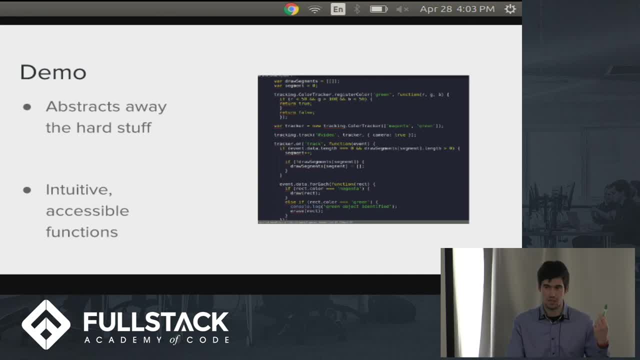 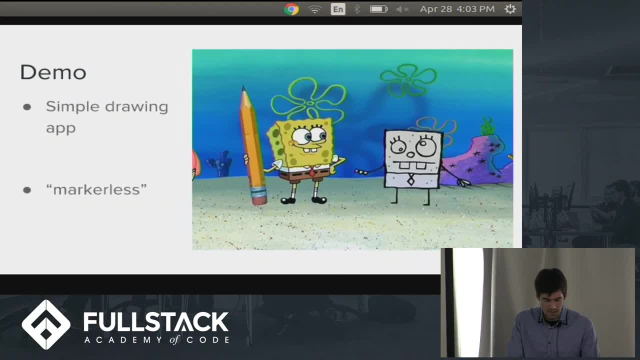 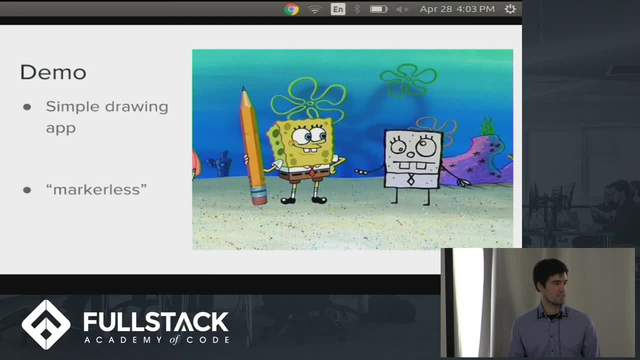 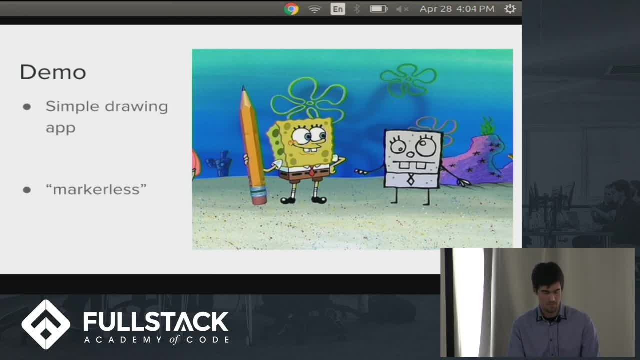 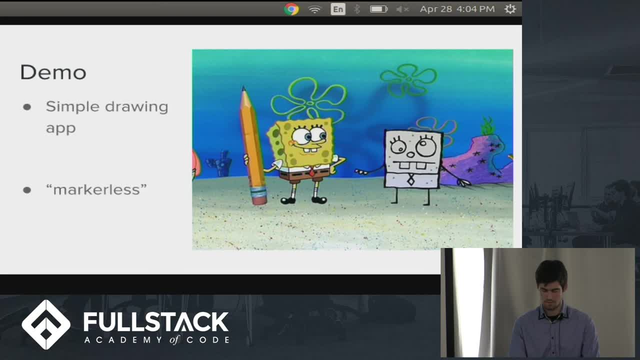 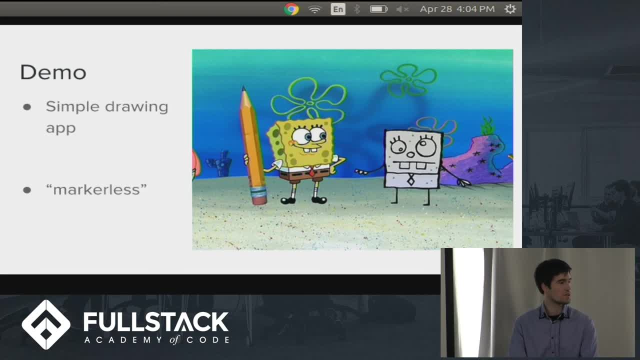 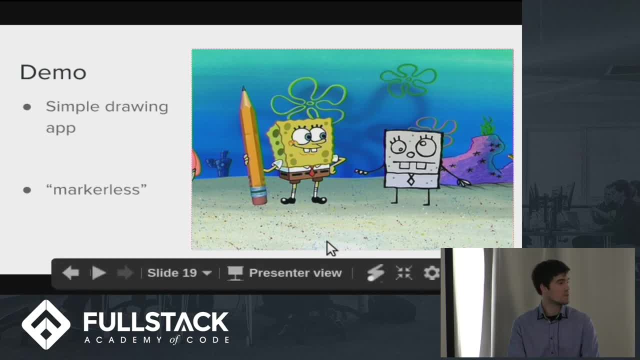 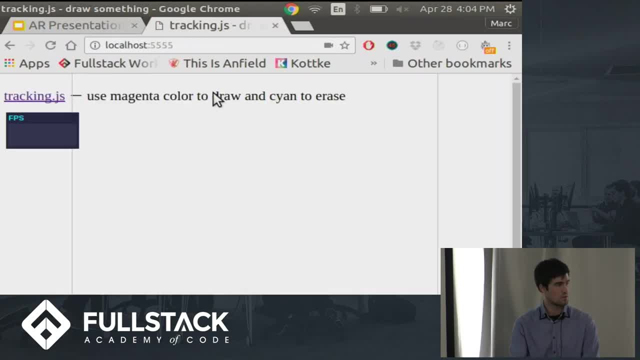 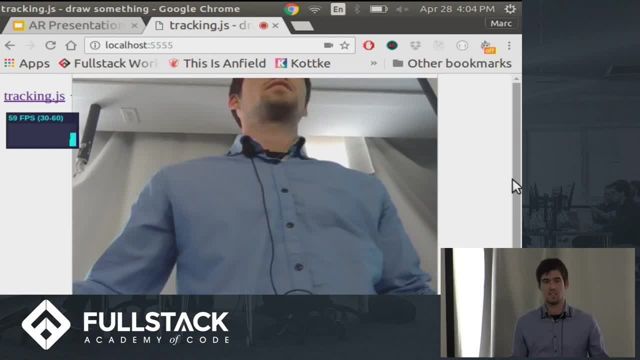 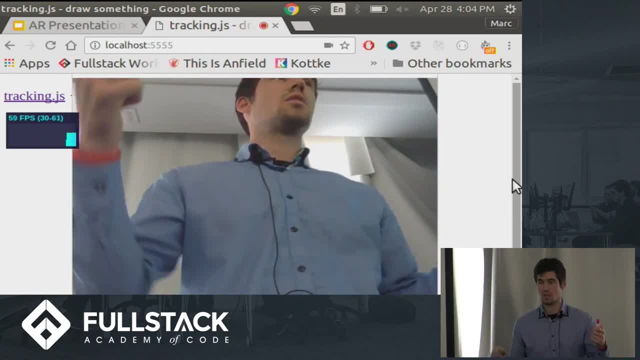 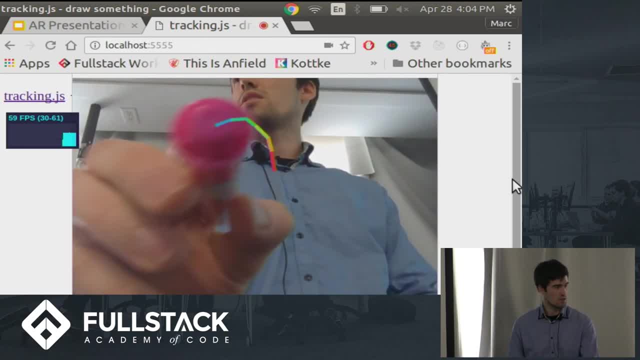 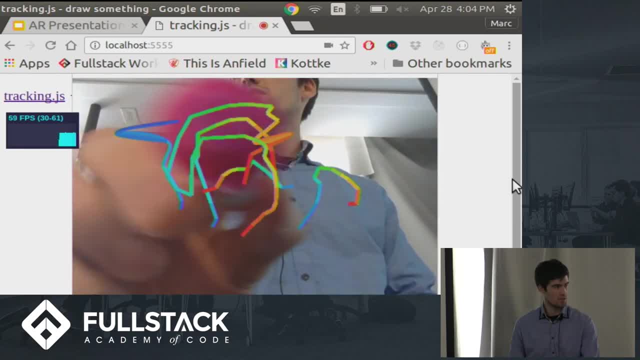 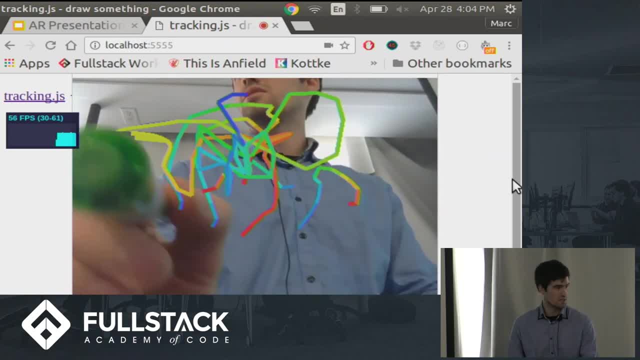 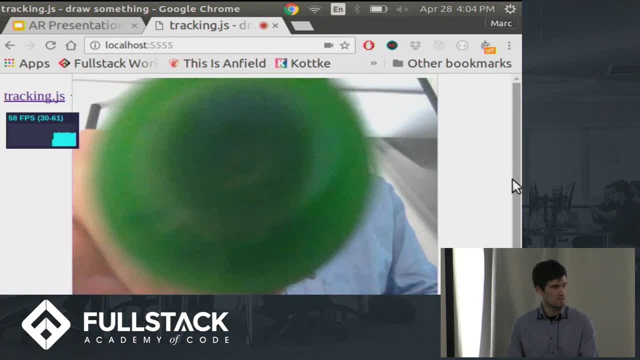 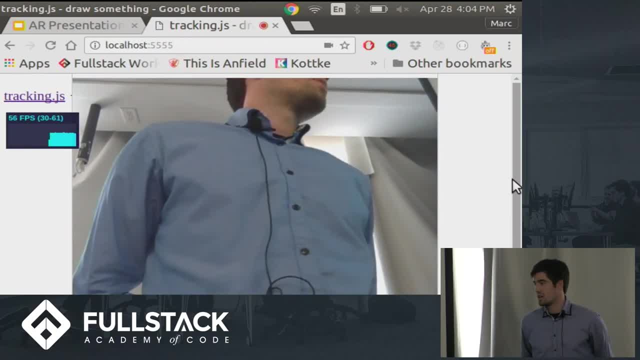 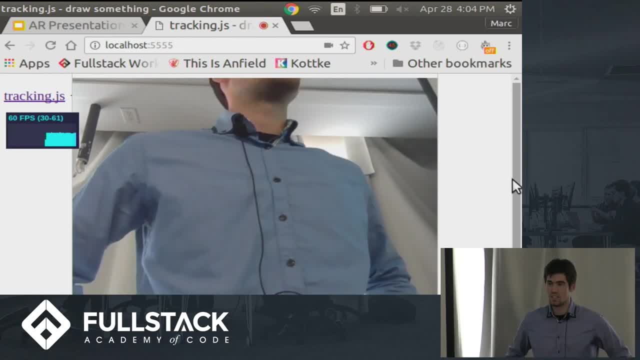 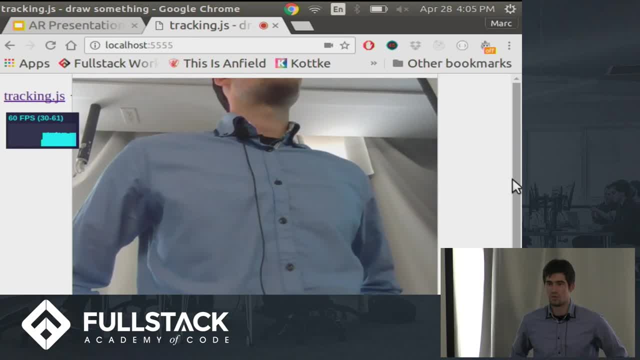 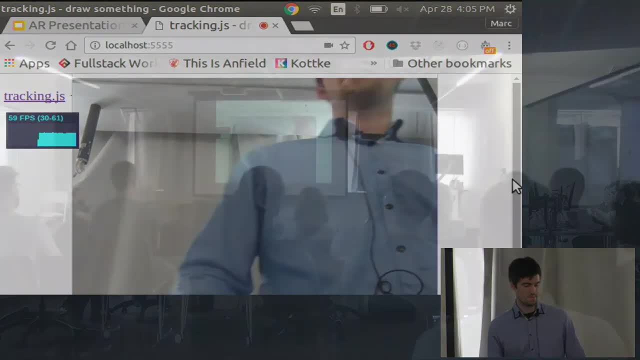